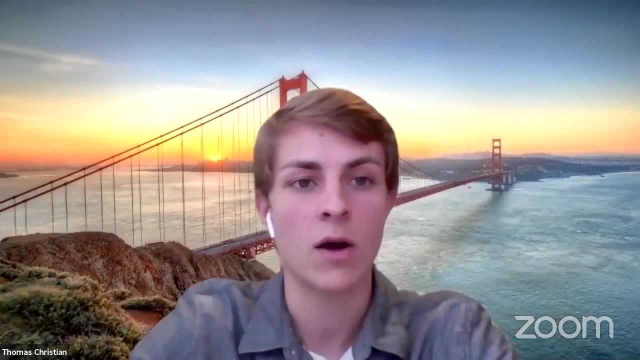 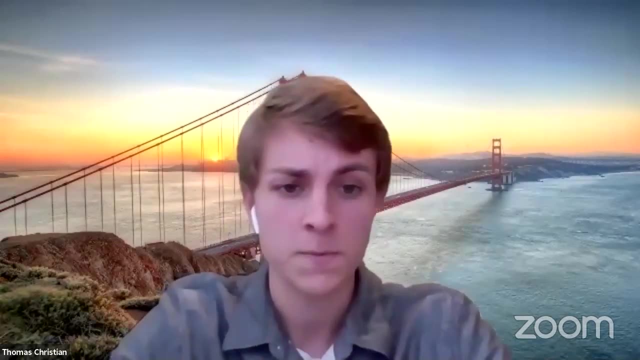 Any experienced data scientist knows that anomalies outliers errors. they happen all the time, and especially during testing, but if left unfixed they can throw off an entire system, And our talk today- sorry, our talk yesterday- was focused on the future of AI. 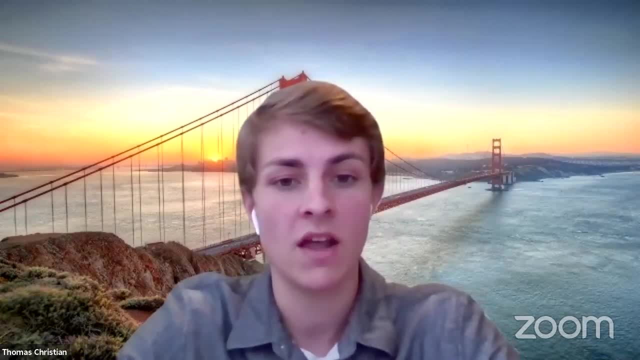 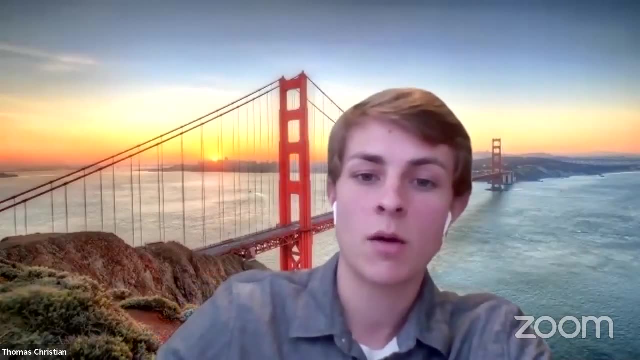 And now we'll take a look A step further and showcase one of our many implementations of how AI can be used in data science. Jay's talk will show us the future of detecting anomalies and how they can be fixed automatically, which could potentially save hours of time, especially with business. 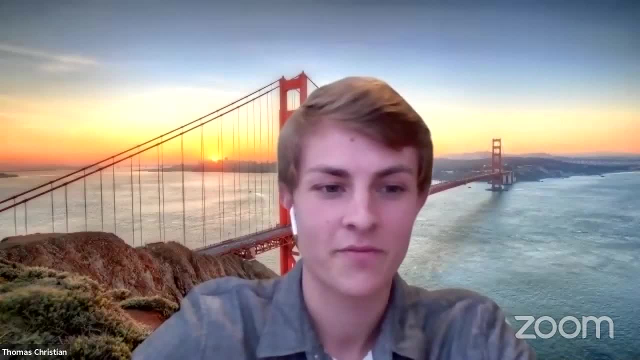 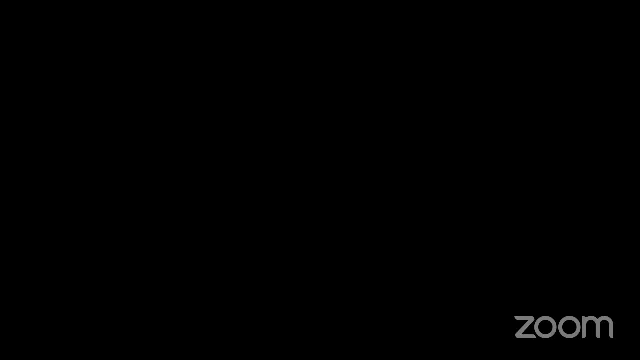 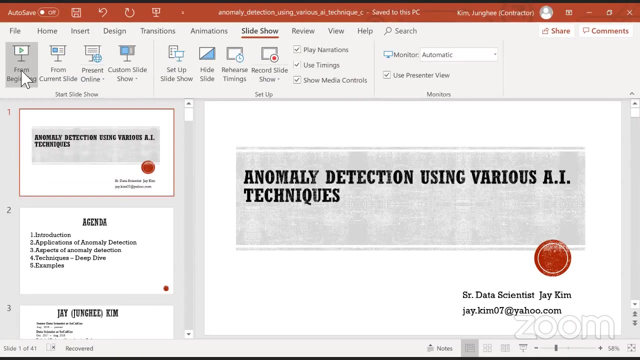 Without further ado, here is Jay Kim. Welcome everyone. Thank you for coming today. Can you hear me, okay? Okay, so yeah, Yeah, we can hear you, Okay, thanks. So yeah, I want to talk about today, about the anomaly detection using various AI techniques. 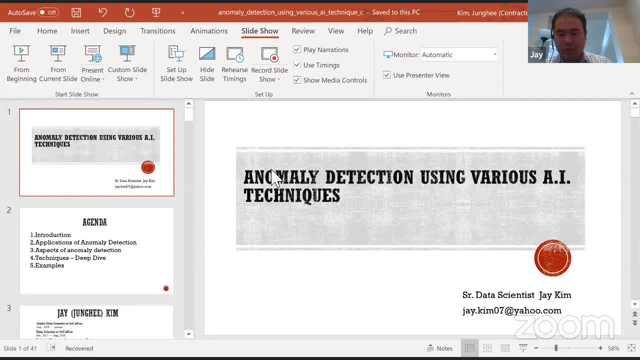 Actually, I have been working as a data scientist for a long time and many of the use cases we have to detect the anomalies, Very oftentimes many of the difficult problems actually so involved with the anomalies. But detecting an anomaly is not that easy. 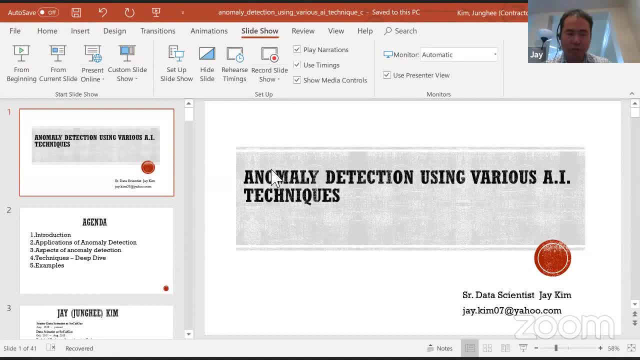 There are a lot of the situations that's going on and we have to understand what kind of business cases and also those situations, And also not only the understanding but also we need a lot of the various techniques to detect an anomaly. That's why the lab is the best for us. 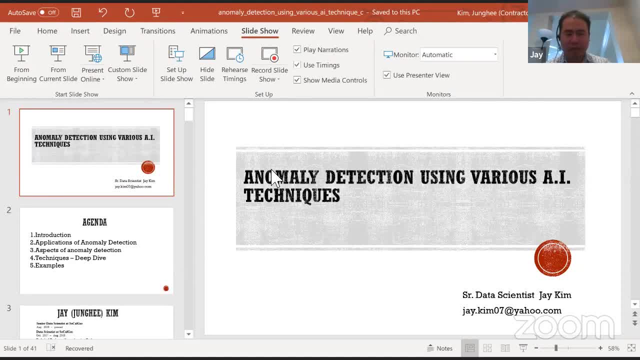 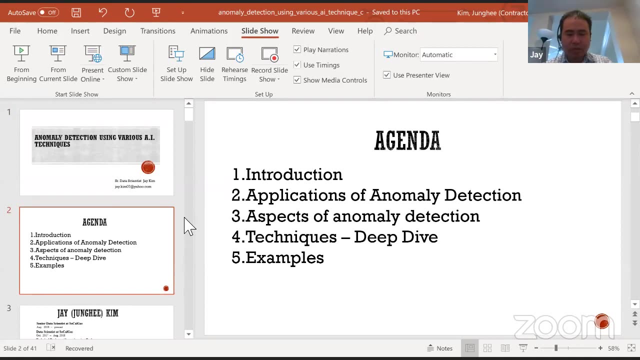 And we're able to do the work and do the job, And we're able to do the work and do the job, detect correctly and also accurately. so today i want to introduce you some very typical and also important ai techniques to detect the anomalies. so today i will talk about the introduction first. 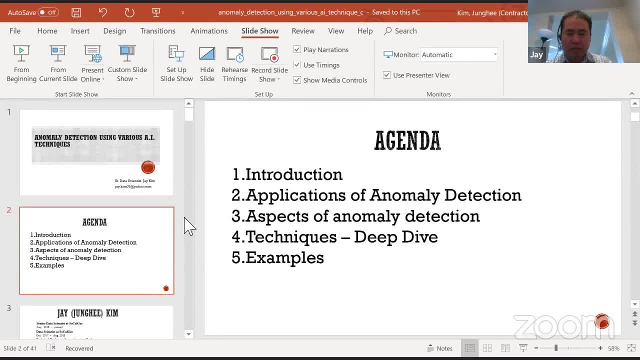 and then the applications and what is actually, what kind of things we want to actually detect, what, what can be actually anomaly, and and then finally, i will talk about techniques. i will talk about some technical stuff here, so it might be a little bit boring, but i'll try to. 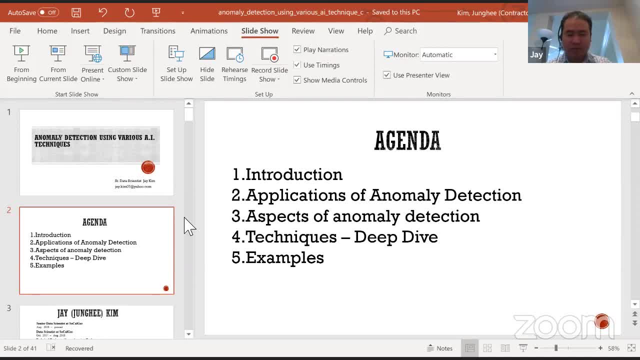 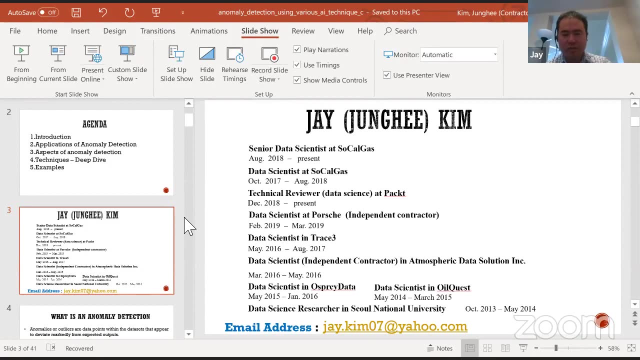 make it more easier, and then i will give you some examples of the use cases and we will finish this talk here. so, before we start, this is me, so i have several- uh like some- experiences, and now i'm working in the socal case as a senior data scientist. 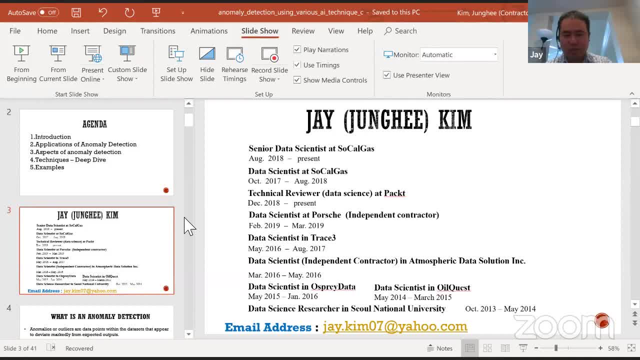 and i'm doing some concert internal consulting as well. so there are a lot of the project is going on and right now i'm working on two big projects and then it's actually in production stage right now. so one of the project is actually anomaly detection also, which is a really uh difficult. but 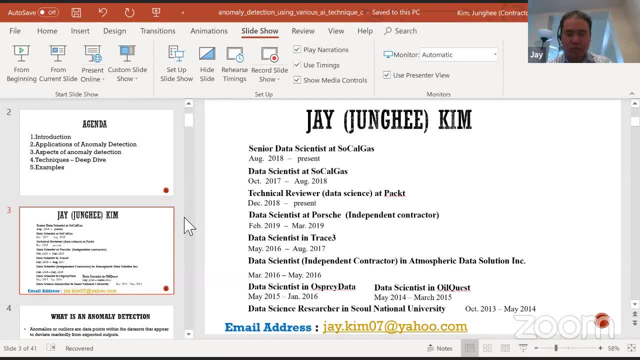 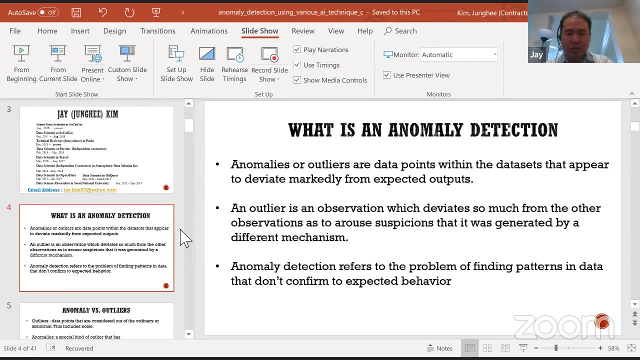 uh, thought, help to me to connect the data to predict the accuracy of the anomaly. so i think with the electron neural network model actually i could be able to manage to detect those anomalies. so yeah, i'll talk about that later. a little bit the techniques. so what is the anomaly? 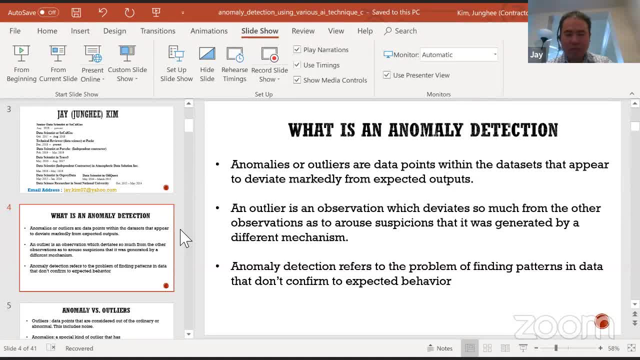 detection actually the anomaly, and before we start actually we need to understand what the animals and what is the outlier. so it's very similar term but it's actually pretty different Neuron Network Model. So outlier can be anything which is abnormal, but the anomaly is kind of something is valuable. 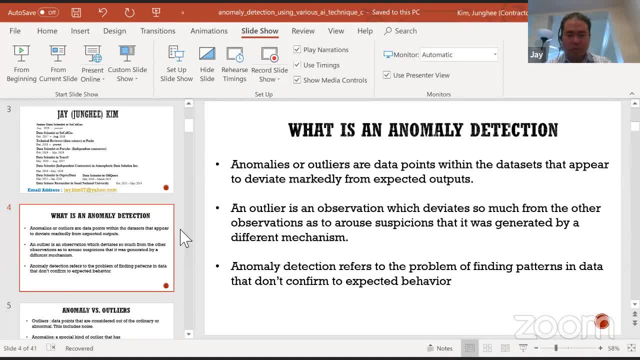 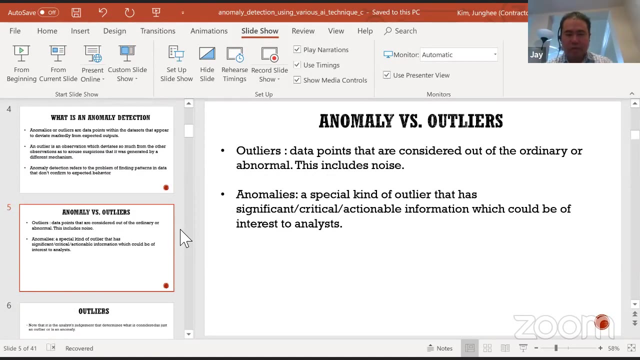 something is actually valuable for business or some kind of work, So kind of anomaly. you can think anomaly is a subset of the outlier, but it's actually more meaningful stuff than outliers. So yeah, this is actually the definition of the outlier and anomalies. 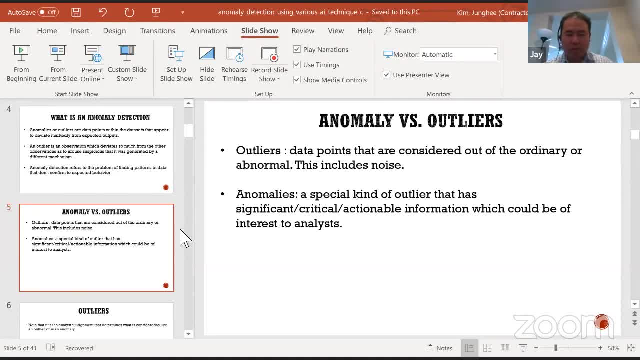 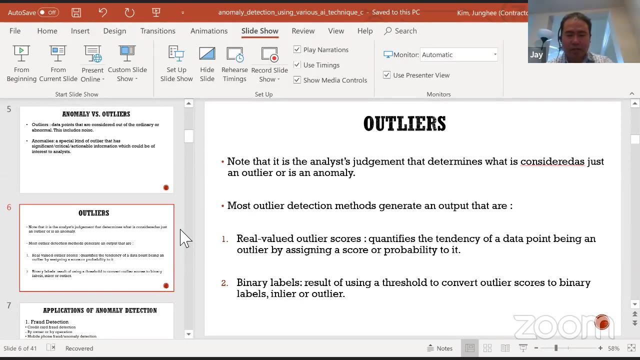 So outlier can be anything which can be actually including the noise, but the anomaly is a kind of a very meaningful outlier which can be good information and which can be actually used in different business analysis. So more specifically about outliers: so most outliers actually can be actually scored. 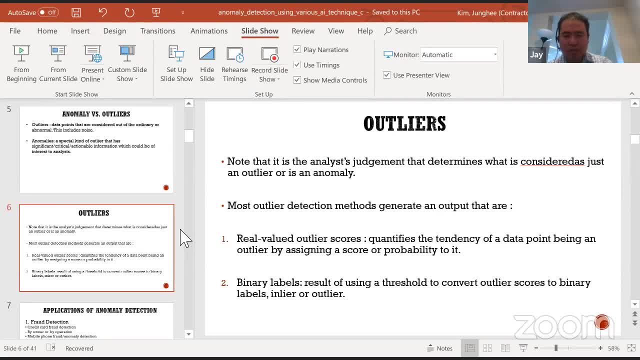 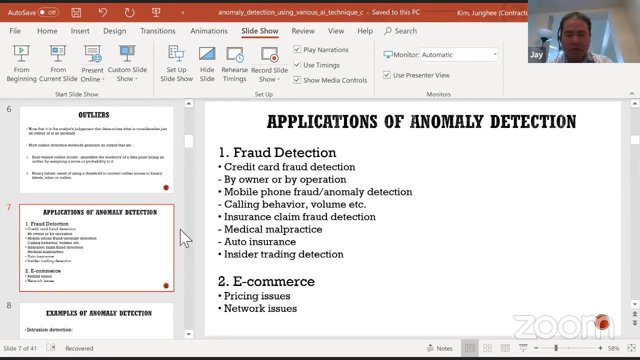 So we can actually score with the statistics and also some probabilities, and there are many ways of the score. And then also we can actually label the outlier as the labels. So we'll talk about that later with more examples. So what can be used for anomaly detection? 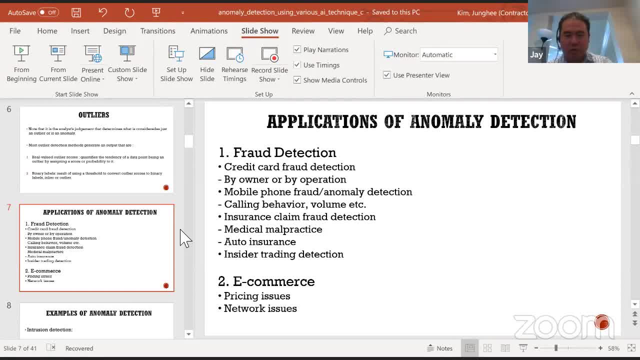 So there are many applications for anomaly detection. So actually fraud detection is actually most common application from the anomaly detection right. So we can actually detect the fraud. credit card fraud- Someone actually can actually fraud, do some fraud in the online or the phone call. 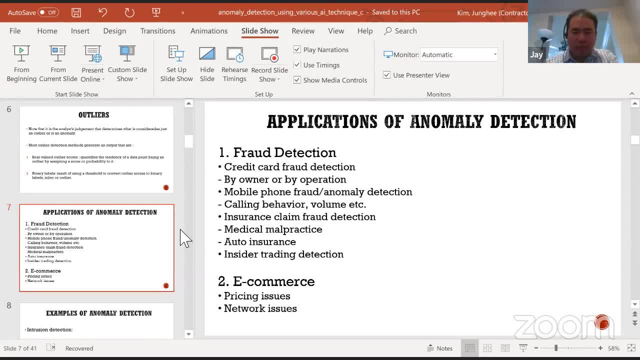 The AI can actually detect it. And then we can actually, you know, actually we can check the behavior of the some kind of fraud calling behaviors, and then automatically by AI, And then there are many medical practice kind of those kinds of stuff can be actually detected as well. 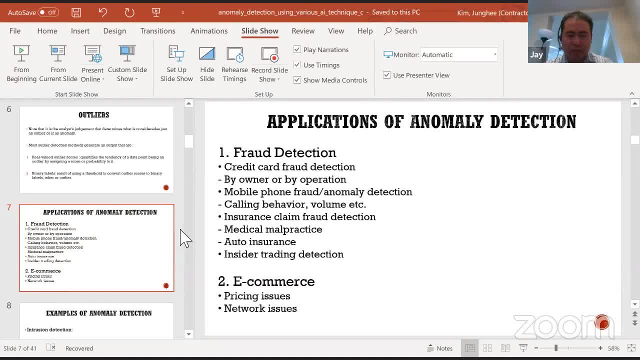 And then there are many different applications like that. There are also another common application is e-commerce, So pricing issues. you know e-commerce, So pricing issues. you know e-commerce, So pricing issues. the working issues actually can be detected. 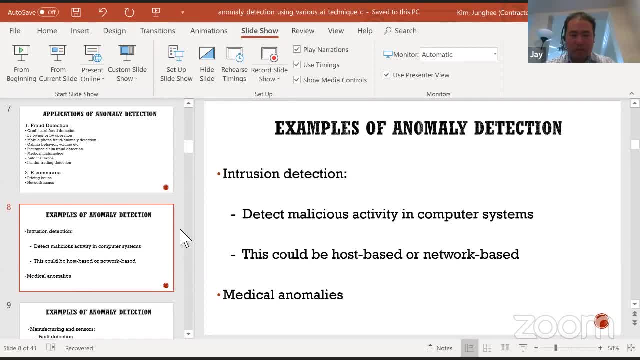 So, and also intrusion detection in the security. And also intrusion detection in the security. actually, some people try to hack, hacked some people's computer, but the behavior is very different from normal behavior. but the behavior is very different from normal behavior, right, So the AI program can actually detect it. 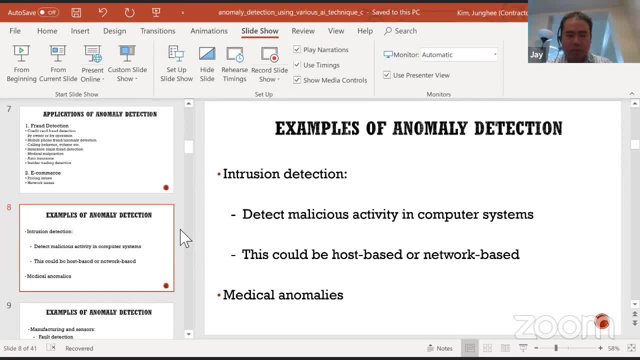 And also in the medical anomaly. So some kind of cancer detection right, And also in the medical anomaly, Aleagui, I forgot. So some kind of cancer detection right. cancers, but the image of the cancer is different from normal, normal people, so from the image they, 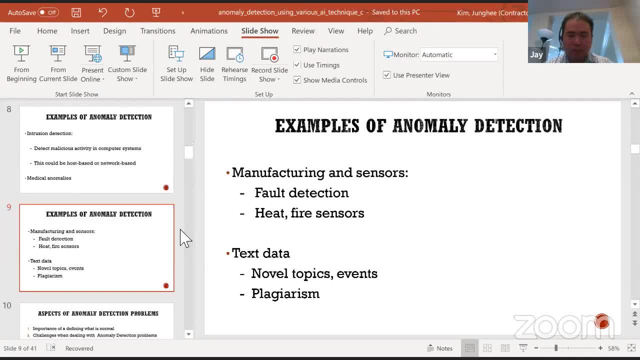 can actually detect the anomalies and also manufacturing and also sensors. so in the iot we can actually detect the different phenomena. so force detection and heat fire sensors we can detect the high heat or fires. and also in the text analytics you can detect the different behavior like plagiarism. right, the novel topics, which is different from normal text, so those can be actually. 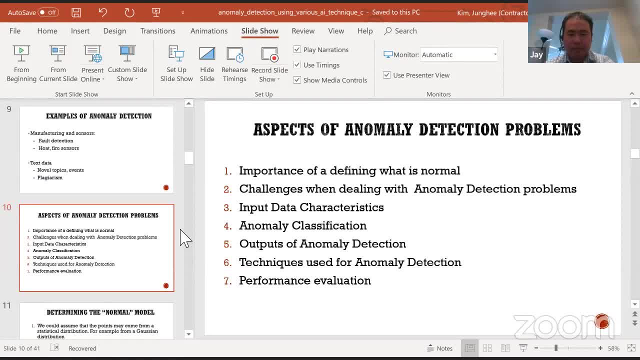 actually used with the ai, uh and also uh. so the aspect of the anomaly detection uh is uh. actually it's very important for i mean many different applications, right, the anomaly session main thing we have to detect. so there are many ways to do that. so, yeah, i will talk about the techniques and what kind of the 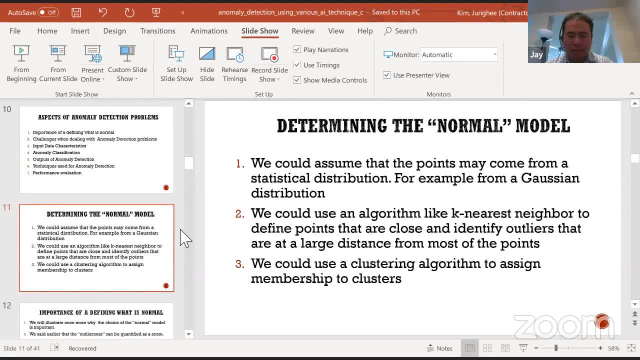 aspect, we, we will need um. so before we actually get find out the anomaly, we need to know what's the main signal and what is not many signal, right? so defining the normal signal is very important. so what can be actually normal? uh, normal signal, normal distribution, uh, and then, which is not the 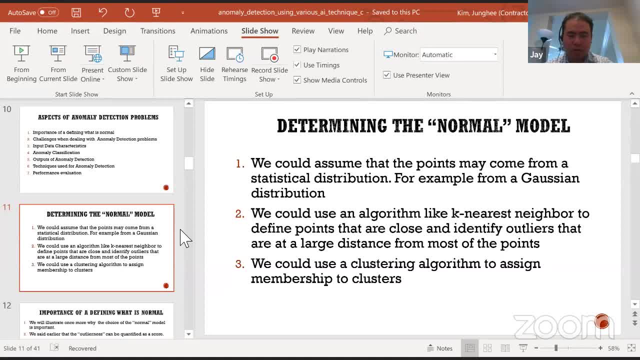 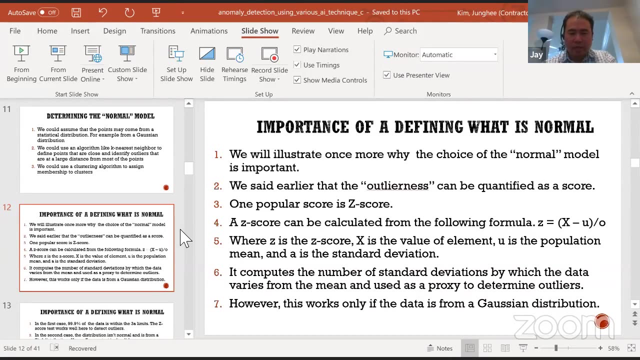 normal dish, like something we don't want, or outside of the what we have, like some main signal, so uh, so for that there are many different techniques, like clustering or k nearest neighbor, those kinds of stuff. so i will talk about that later more. and then, yeah, i will talk about it earlier why it's important, why uh, why uh, defining the. 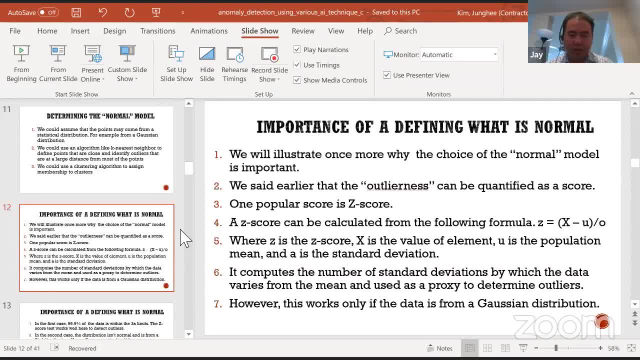 normal signal is important because if you don't, if you define uh wrong, wrongly the normal signal, then that means we will uh actually we will find the outlier or anomaly in wrong way, so it's actually it's wrong from the beginning. so we have to actually find out the normal signal in. 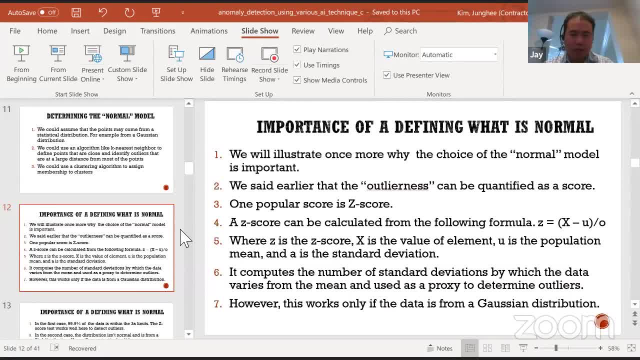 the beginning, right? so to do that, we need to actually see the statistics, like that on this score, or normal distribution, or like key value. we have to see the distribution and then we have to know that what is actually uh main, uh main signal and what we are actually looking for. so this uh. 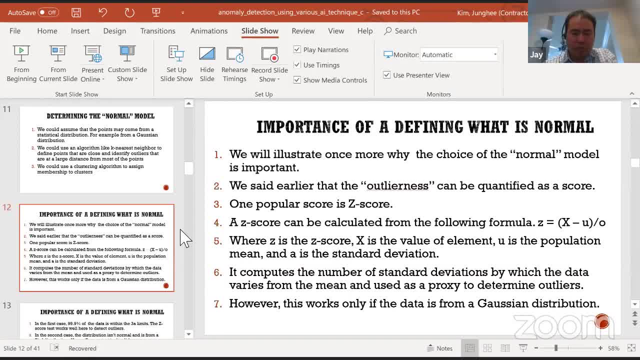 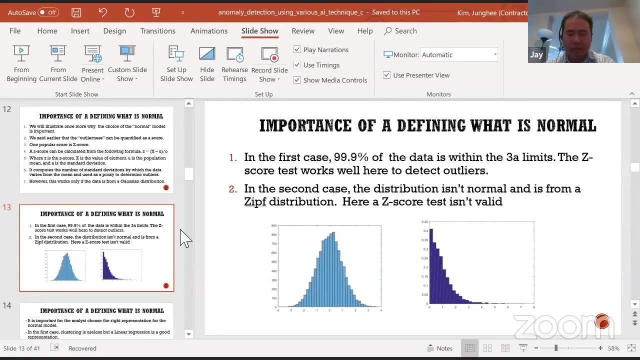 uh, yeah, so this score is one of the popular score, way you know. so, question distribution, another term is the normal distribution. so we, we can actually see that what is actually normal, uh, normal signals, uh, that we are actually uh having main signal, and then also what, what can be actually our, our layers- yeah, this is just a example. so, uh, you can see. 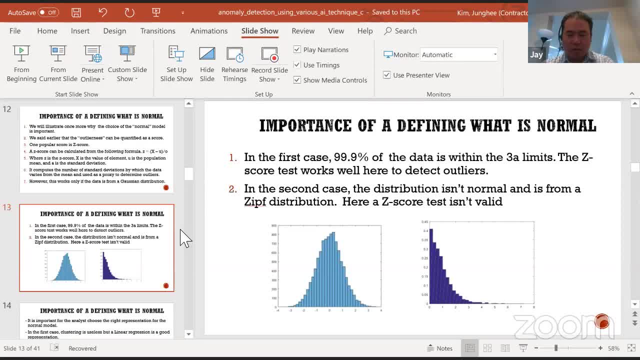 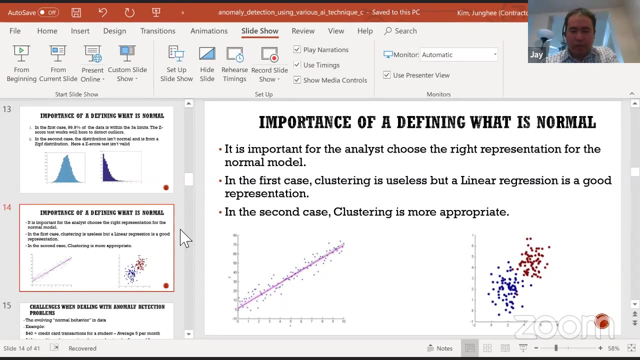 the normal distribution in the left left picture. uh, so most of the signals are in the middle, in the middle of the left side and the right side. uh, in the second case it's, uh, it's not normal normal distribution. uh, so this one cannot be. uh think that way right and then another way. uh, so in the 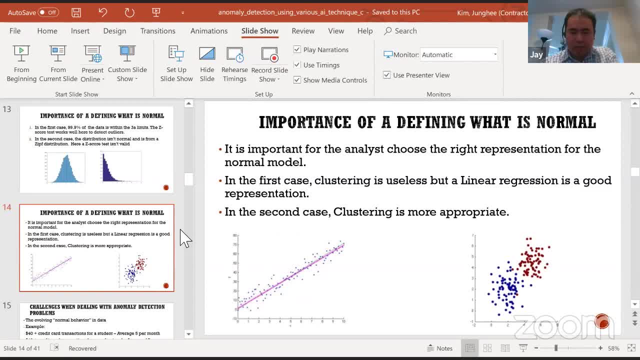 left side main signal is actually in the line regression right, and then the outlier can be far away from the line. we on our term is a model model right. it's a linear model, so it's more far away from the linear is some. it's like we can actually. 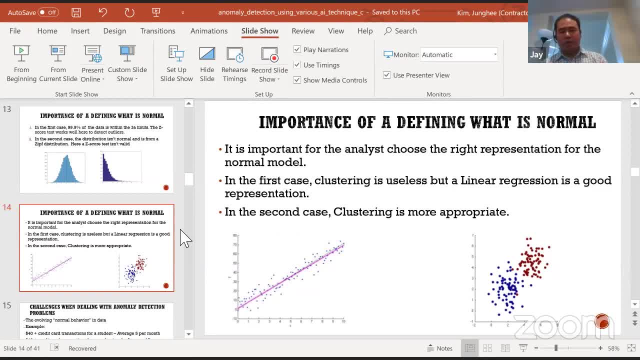 think it's a kind of outlier or anomaly. the left side is a kind of clustering model and we can see main signal saying that it's a cluster but the outlier or anomalies can be spread out. so we can see from this modeling perspective as well, like this: 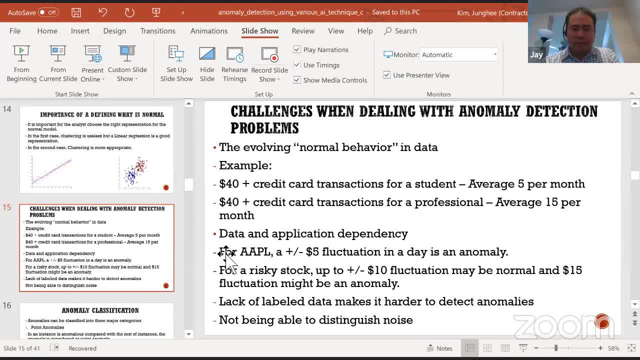 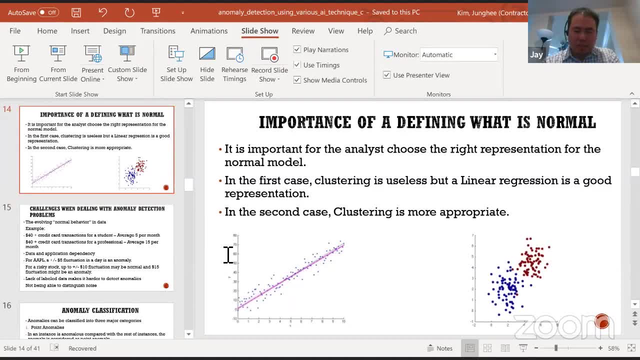 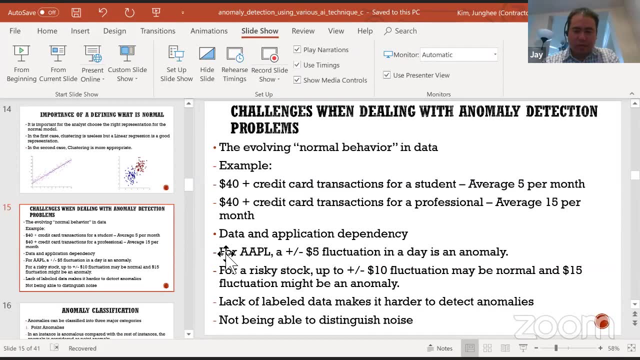 yeah, so it's very challenging because, uh, uh, if a signal is very clear like this, uh, then no problem, but most of the cases, uh, the signal is not clear enough. uh, we have. so there are many uh different cases and also a lot of the different dependencies and and many different, uh, like the noise, noise. 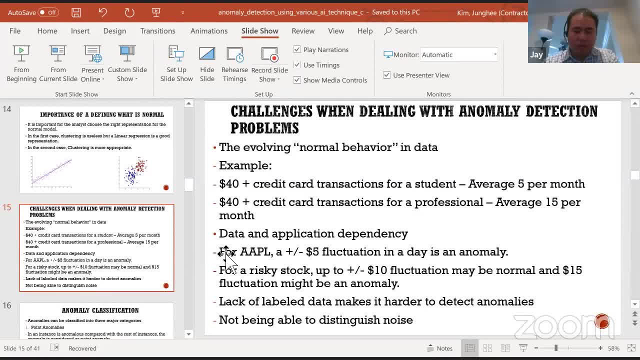 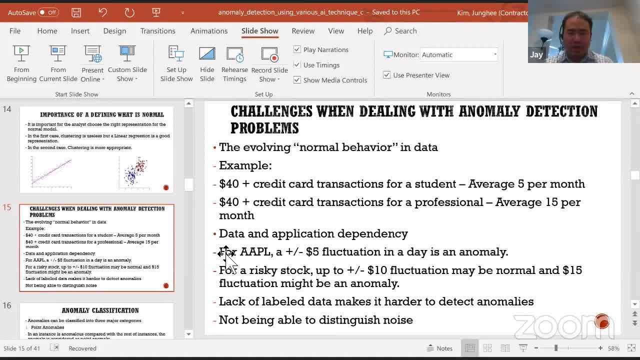 easy. so we have to think about many different problems, and so whenever you actually dealing with the anomaly problems- uh, it's not- you have to actually define the problems first, and then, and then also you have to think about the different dependencies, and and then we can actually go to. 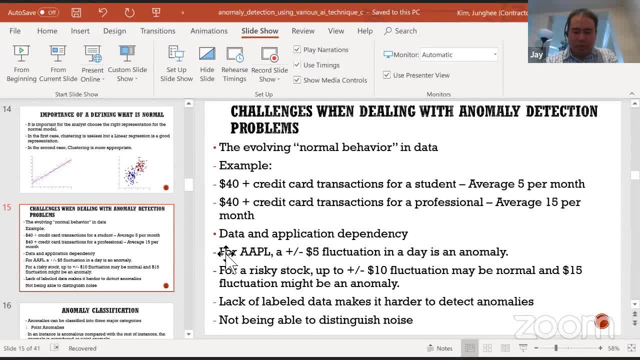 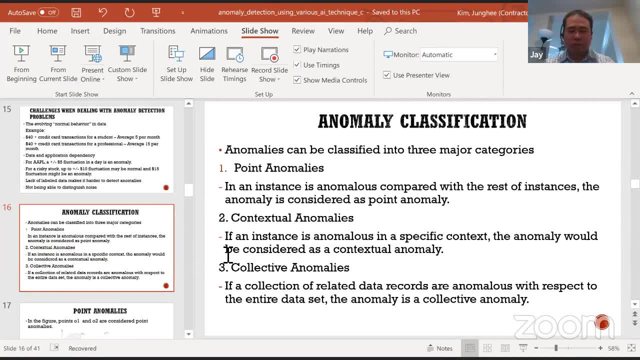 the actual problems from there. but it's not easy, as you can see. so so another way to actually detect the anomalies: classification. i think everyone knows about classification, but uh problem of the classification is that, uh, we need uh enough labels, so without labor we cannot actually classify. uh, but there's another way actually we can actually classify. 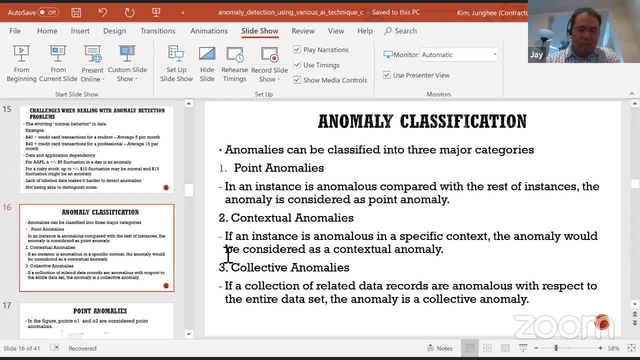 without labels. but but there's a more other way to do it and that's the advanced technique, something like, uh, same as progress learning or or active learning, which actually doesn't require enough labels, but normally actually we need our labels to, to the classified classification. so, uh, for that, uh, the anomaly is not happening very often. 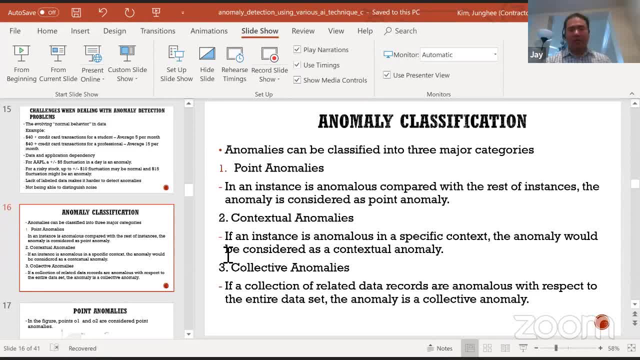 so the label getting labor is not very easy, uh yes, but but it's possible. so i will talk about what kind of the techniques can be applied with the classification here. so point anomalies and contextual anomalies and collect correct anomalies. yeah, i will. i will talk about the next slide. you can see that. uh, point anomalies. 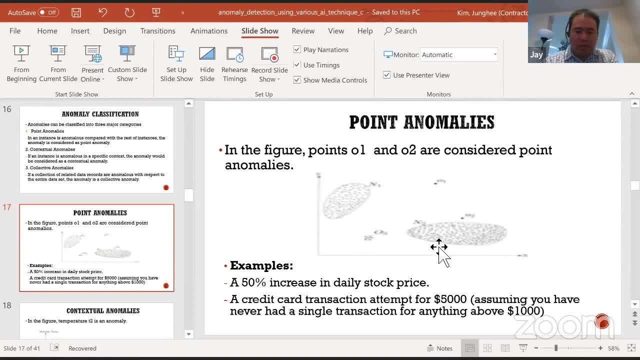 yeah, so we can actually point everything, uh, this like like in the two dimensions كر, but it can be actually three dimensions or different dimensions as well. but you can see some points are actually out of the main plot, right? So we might maybe suspect some. 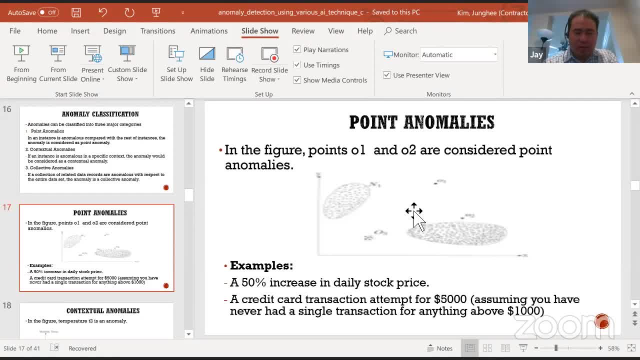 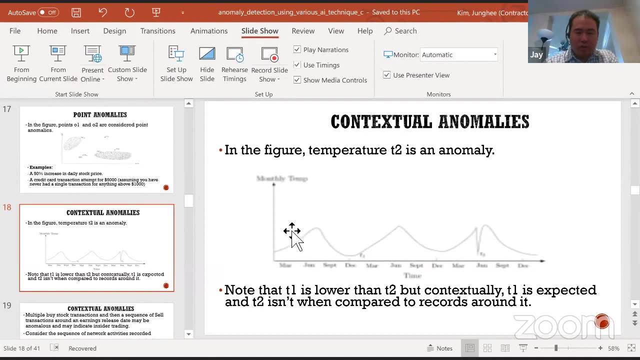 of the like some points as anomalies and then we can actually go deep to that point and we can analyze it if there's really anomalies or not. And then this conceptual anomalies. So you can see, we can also plot this one as a two-dimension, but time is going farther. 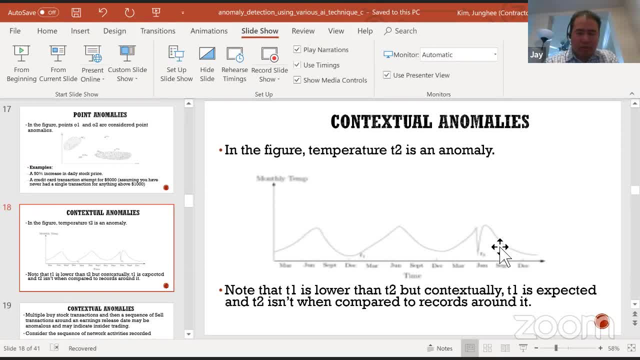 but it's a pattern is very similar, right, But these are some. contact is not the same as the other patterns. So we may be this one maybe because of the anomaly, or we can doubt a bit and then we can actually go in there and analyze this: really anomaly or not. 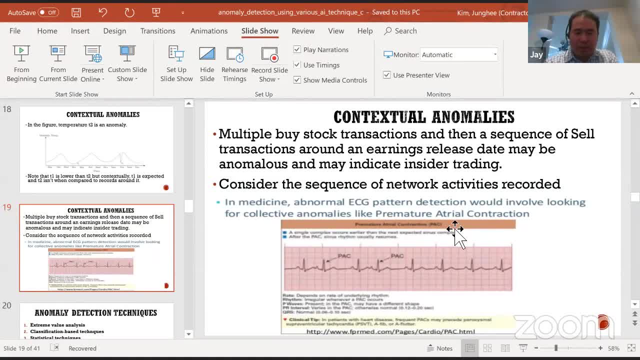 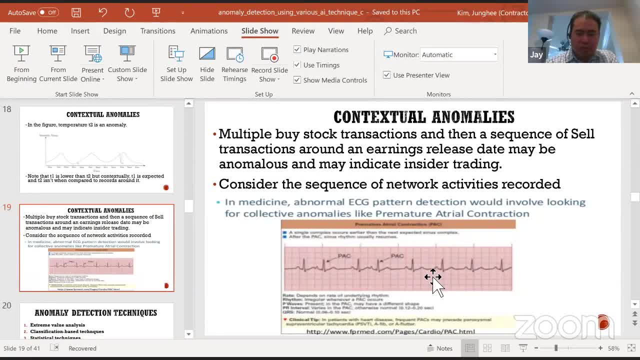 than the same pattern, But for some we can start to doubt that. it's 오� Turkish be even better. Actually first coming out, then the other patterns, So maybe this one might to be anomaly as well, But but we can actually doubt that. but it's not actually clearly you can conclude it. 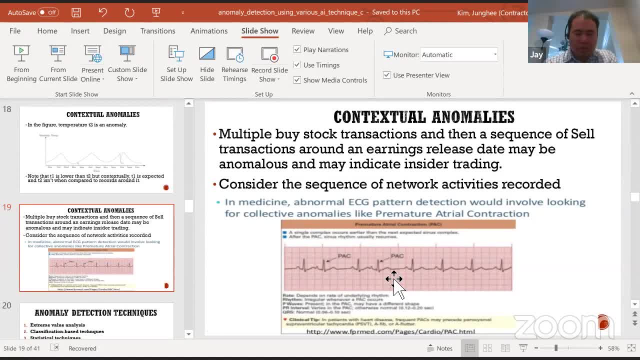 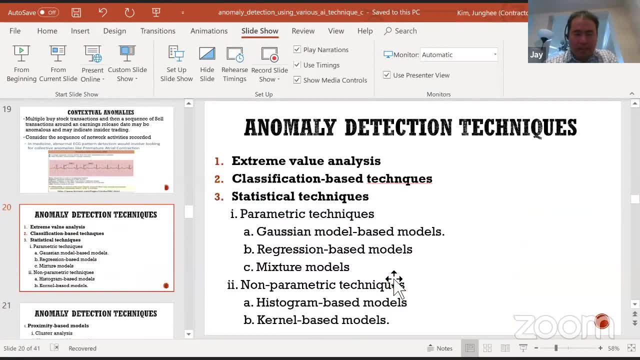 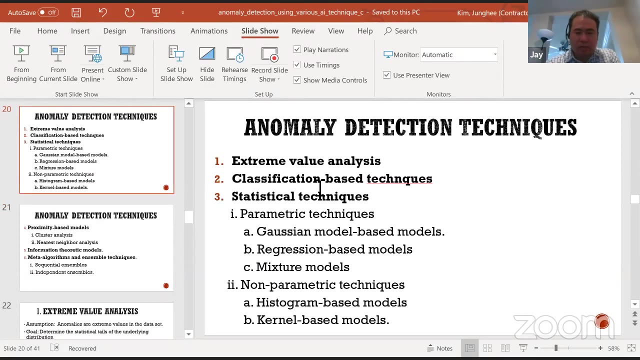 cuz sometimes can be affected by some other factors, So we can't doubt it and then we can go more deeper analysis, were 캣 jeansAN concerns can actually conclude that this one is clearly anomaly. Yeah, so I actually summarized some of the anomaly detection techniques, from one to six. 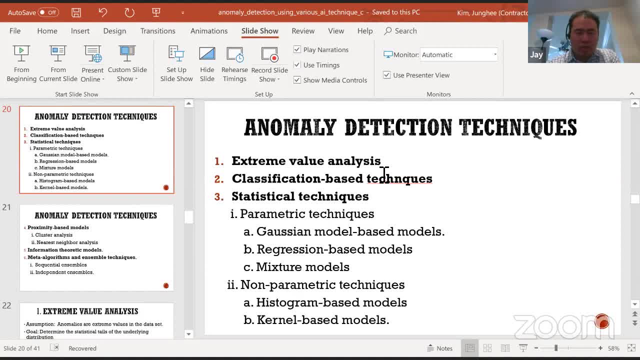 So one is the extreme value analysis. So some values are very different from just a few values, are very different from main values. Then maybe they can be actually anomaly, anomalies, and also secondly- I chose to leave earlier- classification can be actually help. and thirdly, you can actually do some statistics. 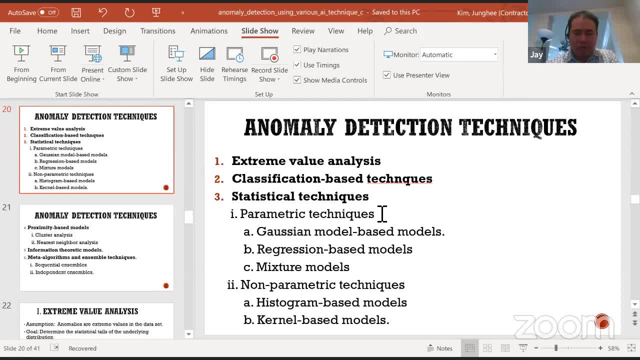 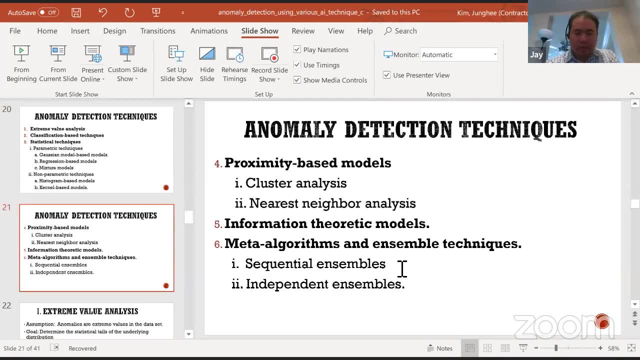 Maybe we can use some statistics to detect the anomalies- There are many techniques, So I should talk about that a little bit later- And proximity based models, So the clustering model or nearest neighbor model- you can actually detect the anomalies And information. theoretical model, something like a p-value- p-value is 0.0, I mean 5%. 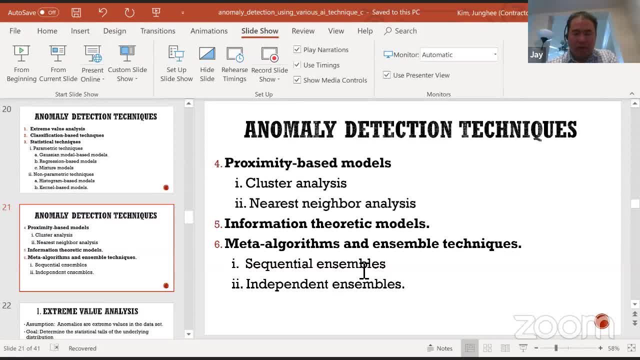 out of the order or the distribution of the values. We can say it's a significant or not, those kinds of stuff. So there are many different statistics which can be used For our layer detection, and also meta-algorithms and ensemble techniques, something like a. 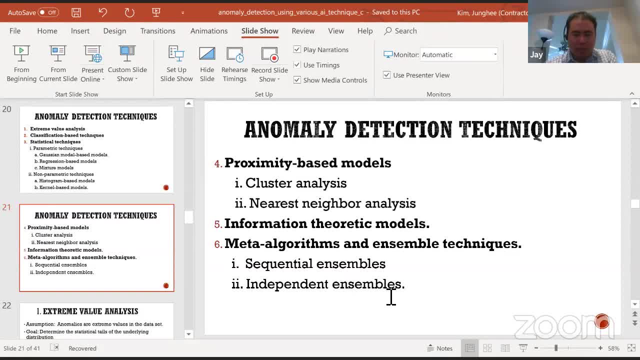 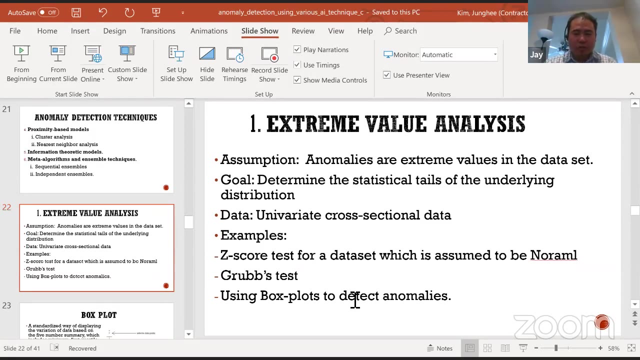 sequential ensembles or independent ensembles. So this one is based on the time, but this one is not. something like the random forest or XGBoost can be actually detect. some some way we can actually detect the anomalies. So yeah, let's start with the extreme value analysis. 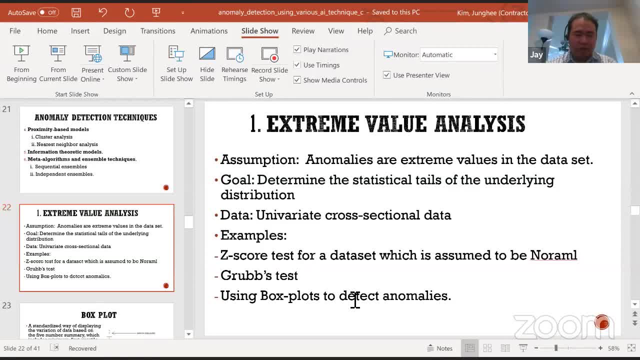 So the anomaly can be extreme values, So very different from all main signals. So to detect that we can actually we can actually use some graph or get some tests with the SGS score or go up testing some box plot, something like that. 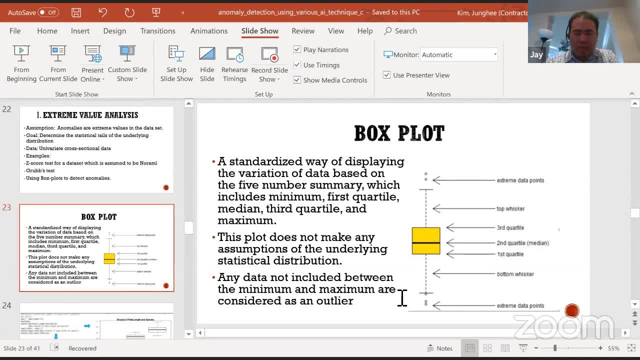 So So one example, so box plot, So main signal is mostly near the mean value, And then after quarter and this max value, and this is a minimum value, But the outlier is actually out of the max and minimum value. So this we can shoot out as our layer. 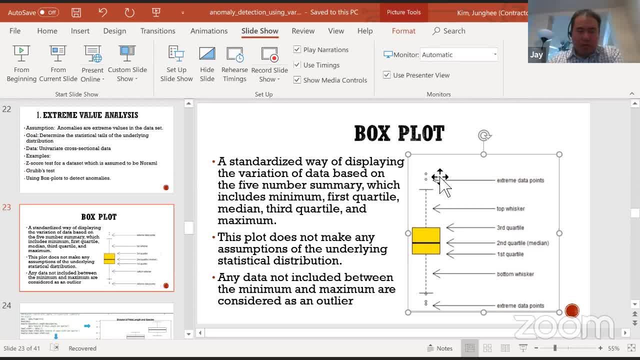 But the outlier doesn't mean it's an outlier. But the outlier doesn't mean it's an outlier. But the outlier doesn't mean it's an outlier anomaly. So we have to think about what can be good for the business. So we have to analyze more. 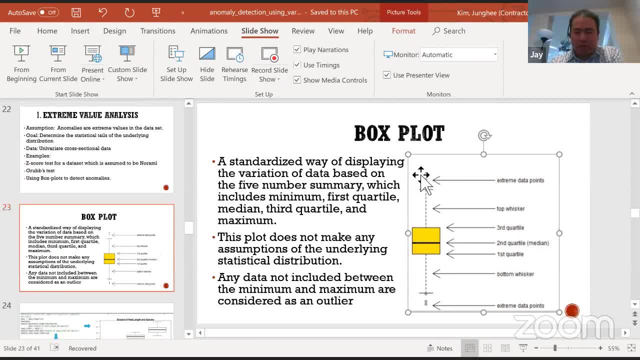 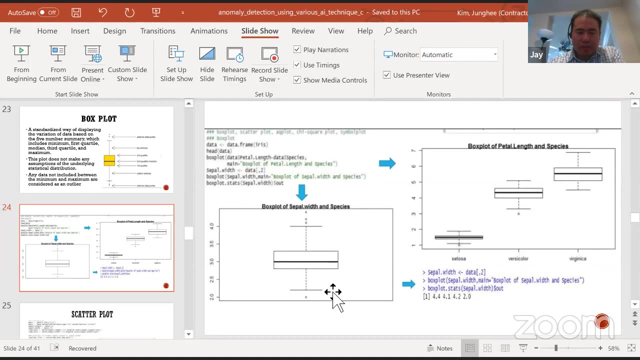 to verify this is a real anomaly or not. or it can be actually noise, So we have to be careful on choosing this as an anomaly or the alliar. So this is another example. So this plot is only one variable, but this one. you can see that several variables, several features can. 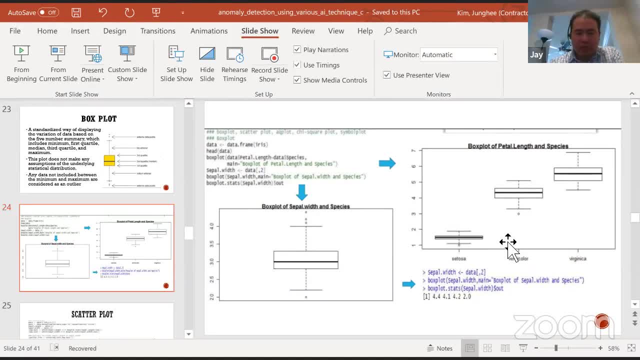 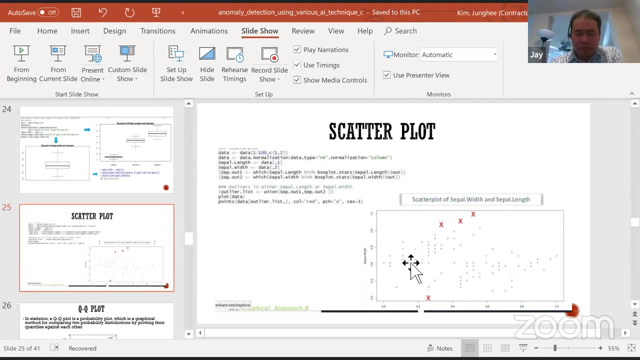 be. actually we can detect The several features the alliar is each, and then we can actually verify those anomaly or not. And then two-dimension- same thing- main signals actually stick together and then the alliar or anomaly can be actually out of the main signals. So we can actually 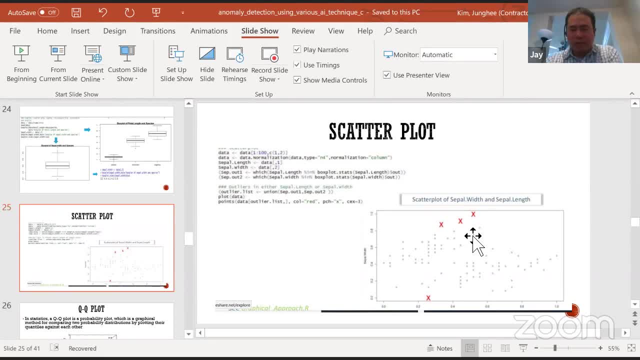 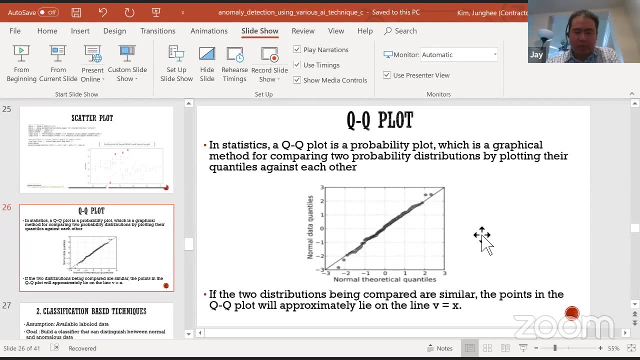 doubt that it's an anomaly. But again we have to be careful. This is whether we choose this as an anomaly or alliar. Then Q-Q plot is a little bit different. So you can see that it's a normal theoretical quantile. So that means it's a normal distribution. And then this is: but this is a theoretical. 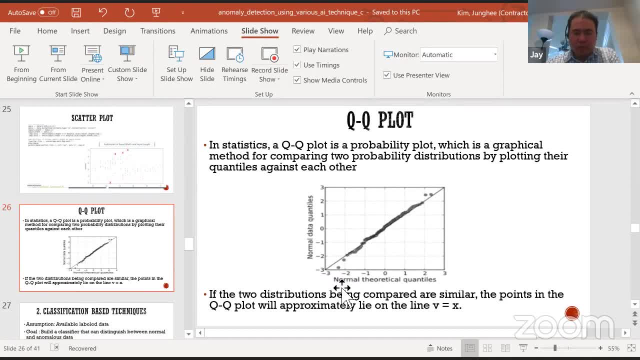 So it's a kind of we choose a normal distribution closest normal distribution to the quantile distribution, and then this y-axis is an actual value. So we plot that as x-axis and y-axis and plot it, and then if some point is actually out of the main line, that means 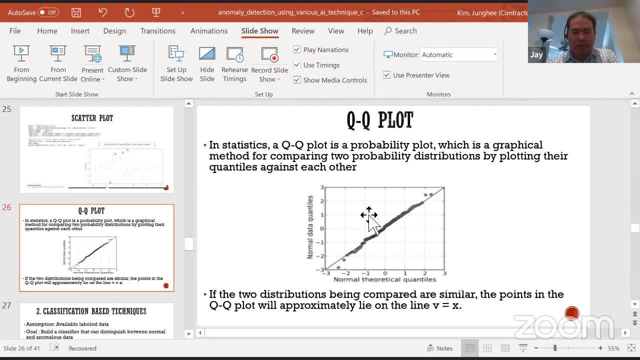 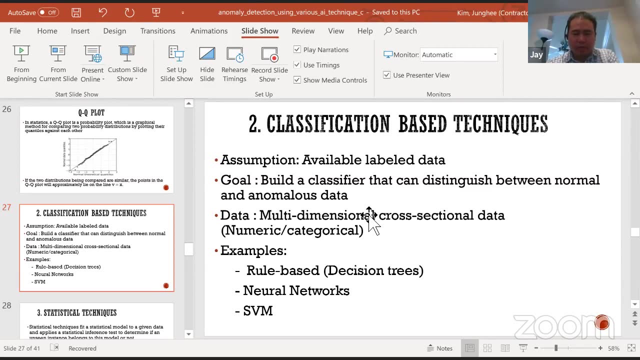 that can be actually an outlier. But again, the anomaly is a little bit different, so we have to be careful. If we think there is an anomaly we have to go more further. Then classification: I explained earlier a little bit. So there are many different ways of the. 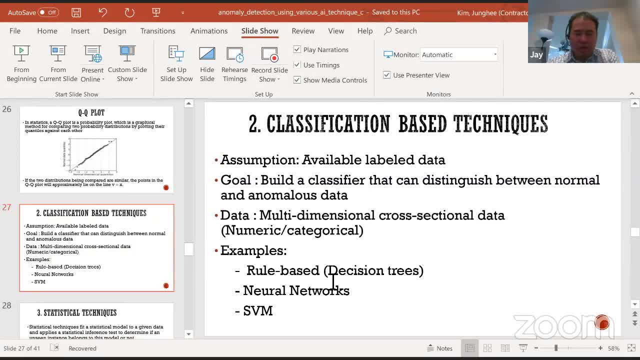 classification right. So rule bases, typically the decision trees and neural network. Nowadays it's very popular, Many companies or work projects. neural network is more like very, very accurate in some way. but you have to have a enough data, you know. So computer power. Then SVM is another way. So it's an Eugene Conrad trick. 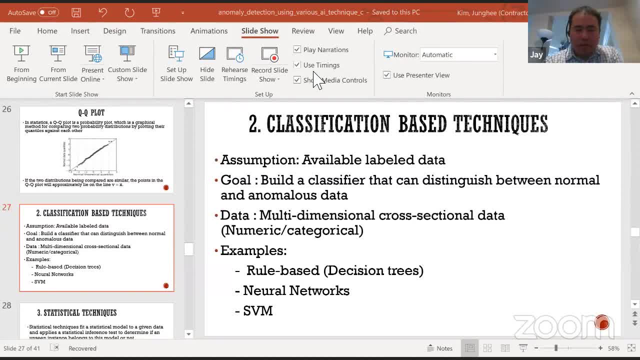 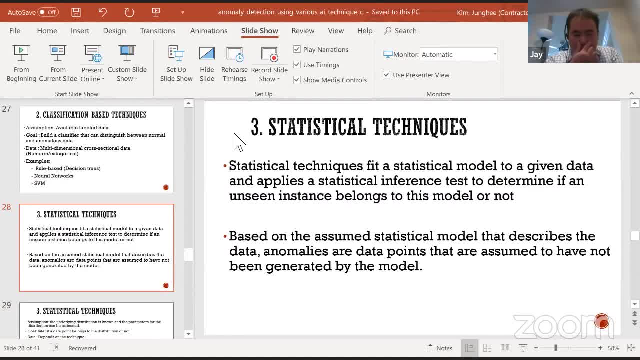 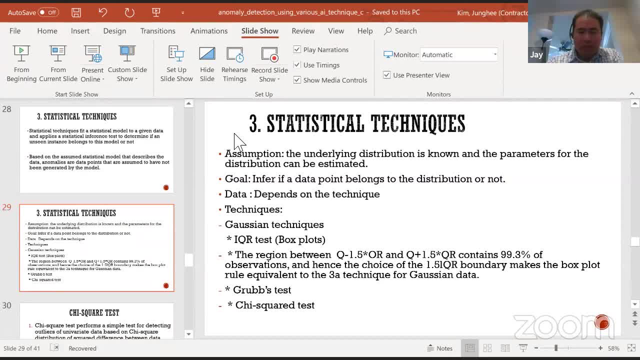 ways. that's right. so, yeah, there are many different ways, so try. squares test is a very typical way to check the significance of the data, and group test is similar. and then i was mentioning about the box plot. yeah, which. so which is a more think about the calcium distribution, and 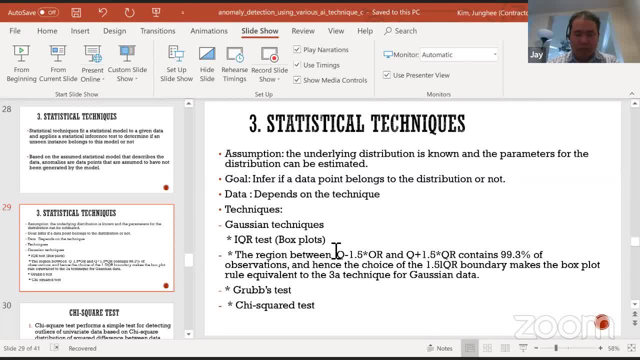 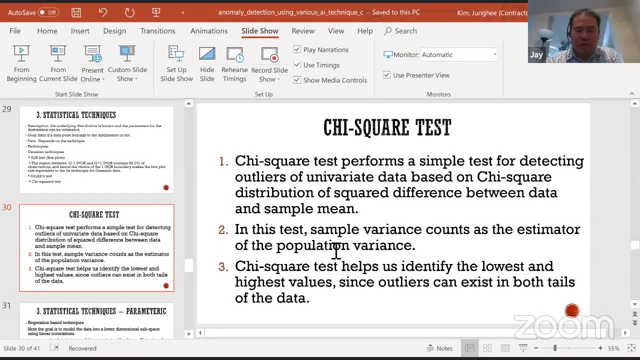 and then you can see the site as a outlier. yeah, so this is, uh another example. so i think everyone knows to try square test. so, uh, we are, we want to see the uh uh which is a significant or not, right, so we can actually check the p value. and it's a more less than 0.05, then it's very significant, uh, but but if it's not, then 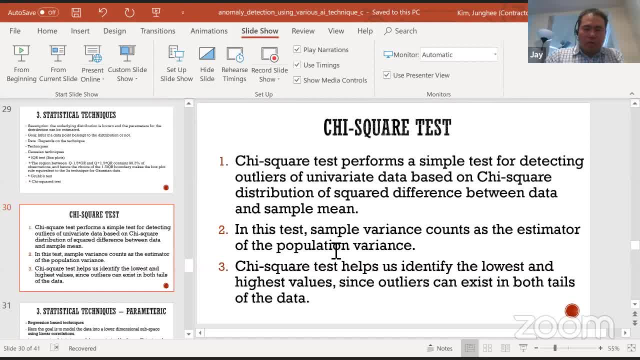 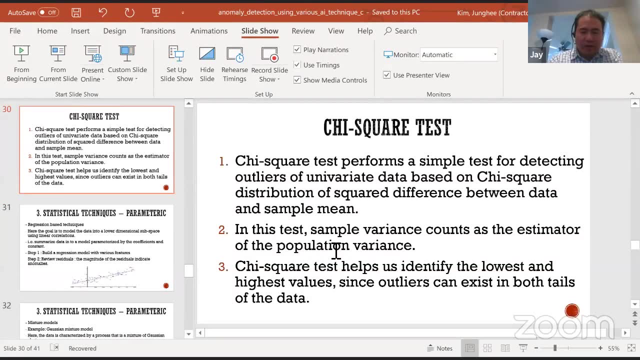 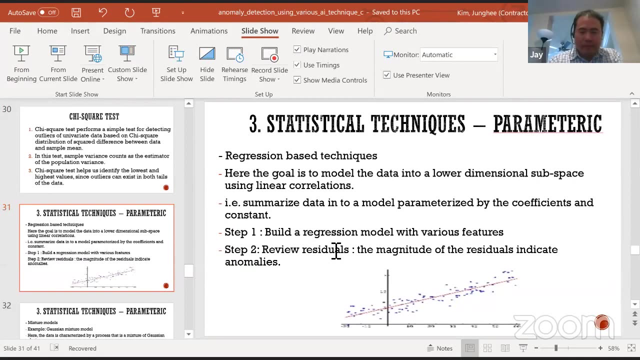 it's actually not significant. so we know, uh, what is actually? uh more, more significant or not? if it's not significant or more, uh mean mean values. also very variance count and population variants can be used now and then. yeah, i was explained that a little bit earlier. regression can be another way, so 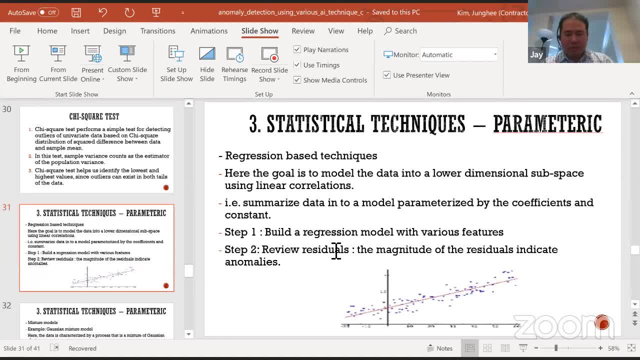 the, the outlier or anomaly is out of the lines. uh, it can be actually a linear regression or non-linear, depending on what kind of model we are using based on the actual data. So the residual is actually a more higher residual. We can think it's more outlier. 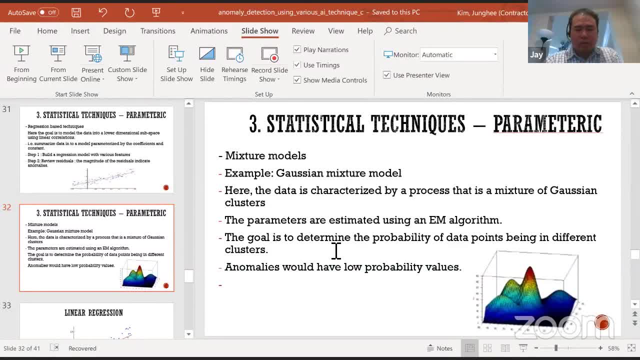 And the mixture model is a little bit different concept. So Gaussian mixture model is actually checking all the Gaussian without the actual value, The actual data. we are actually matching with all the Gaussian. For example, if there's many different features, let's say five features- we actually make the five Gaussian distribution matching. 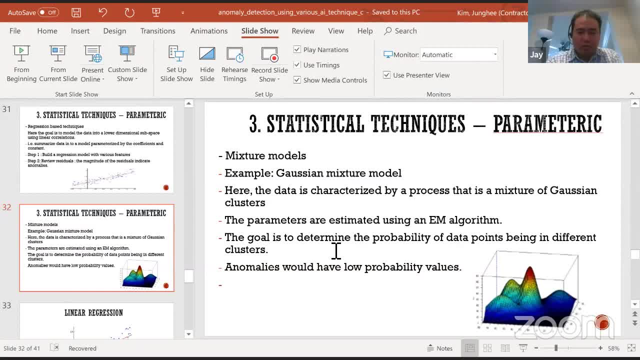 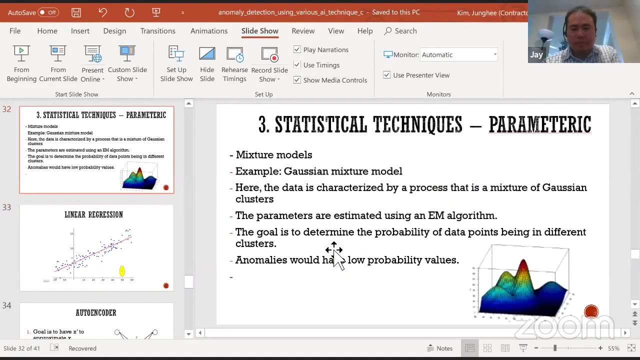 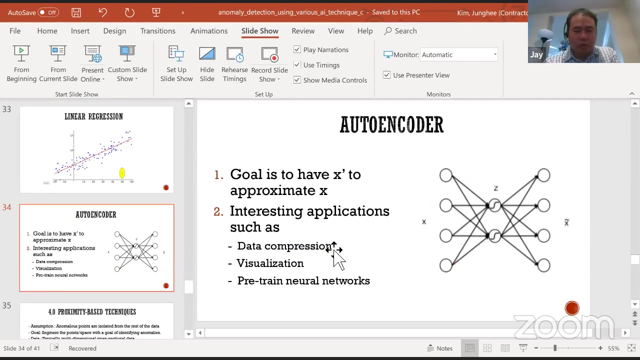 And then we try to map with the actual value, with the actual variables, with the different Gaussians, And if some data points it's not fit to the model, then that means it can be outlier. And there's also autoencoder. It's another thing we are very popularly actually using nowadays. 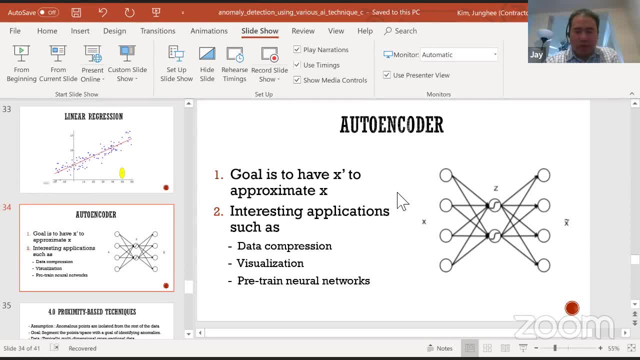 So autoencoder is a type of the neural network. So the X in the beginning, the X layer, first layer, is the actual data And then in the middle layer we call the Z value, which is the compressed representation of the data. 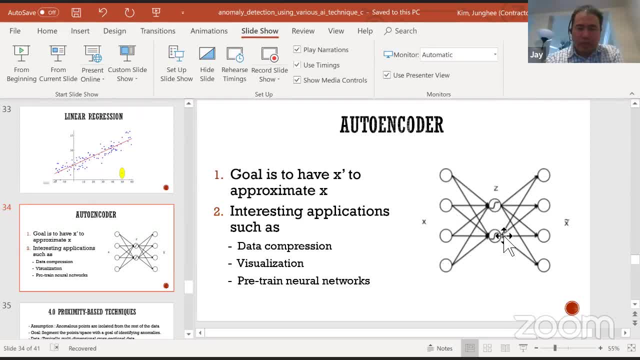 So it's actually four node And then the middle part is the two node. That means it's compressing the data into a latent space And then after that the data is going back to normal. So this is generating the data back to the output. 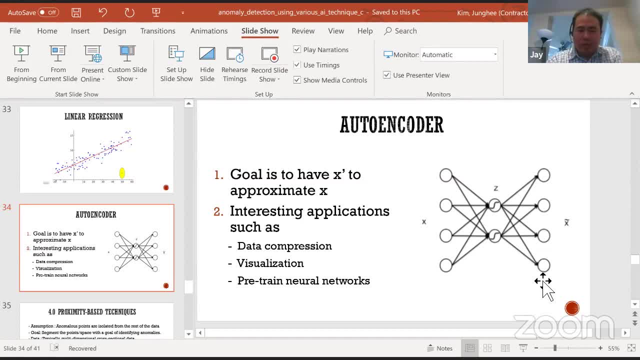 So we call this one as generated of the data, which is the approximation of the actual original data, And then also in the latent space we can actually check the different way of the approximation, So this kind of the, and then we can see the representation of the middle layer. 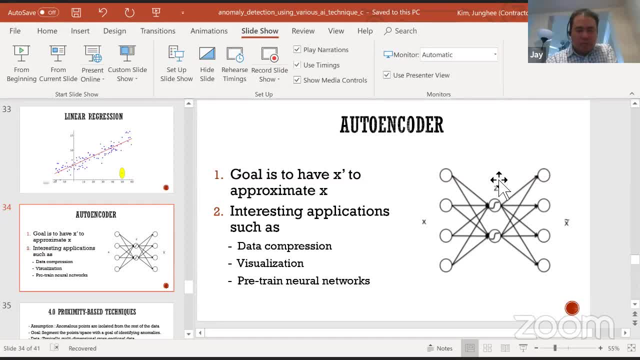 If some value is not from the is close to the main value, I mean we can doubt it as a outlier as well. So there are different way of the application for this model. But yeah, I will just. I just explain very briefly here. 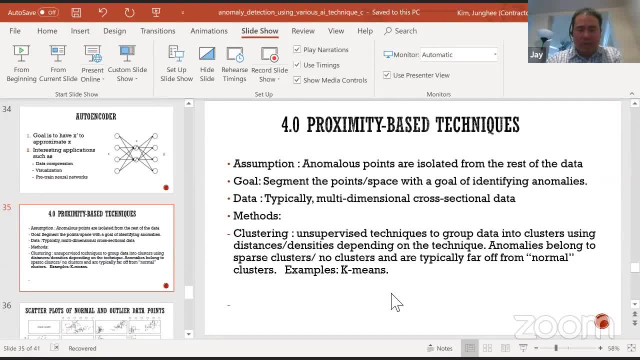 Proxima multi-based technique is similar. So if it's close enough, then that means it's close enough to the main value, then this, this main main data set, but it's out of the main main data point and it's far away than this outlier or anomaly. 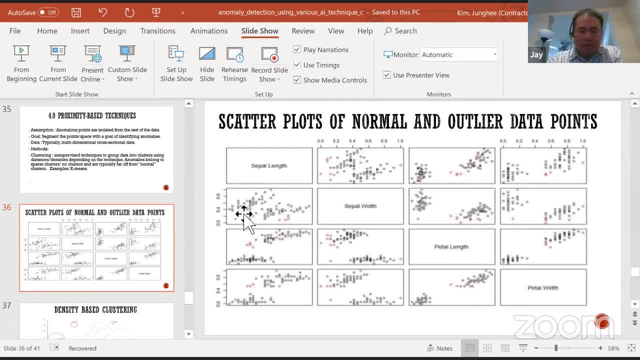 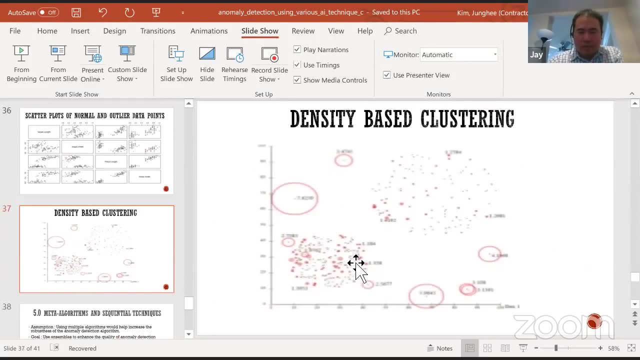 So yeah, this one explains very easy. So some data set, some data are out of the main main point. So you can see it's it's not really a main data but but we can doubt as some outlier And also density can be. 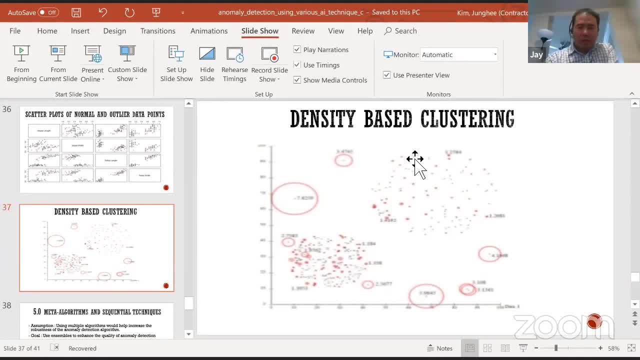 can use a density of the data point. So data point are in very dense, Then it's a main signal, but it's very sparse We might think as maybe outlier. So but yeah, or again, anomaly can be a little bit different. 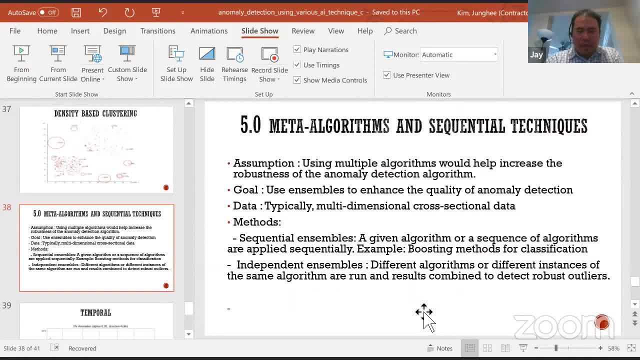 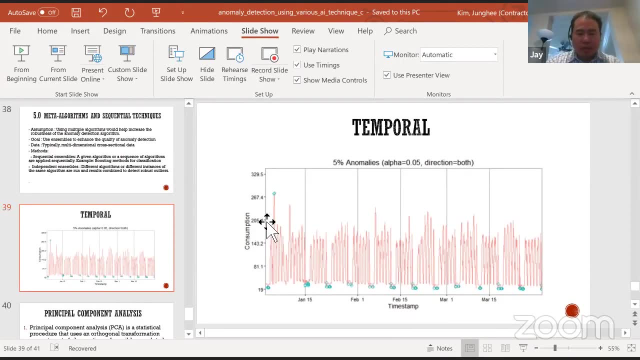 So we have to analyze more further. Yeah, And then this one so time. I think I already explained this already, right, So we'll go over. Yeah, So in the time series you can see that some value is out of the. 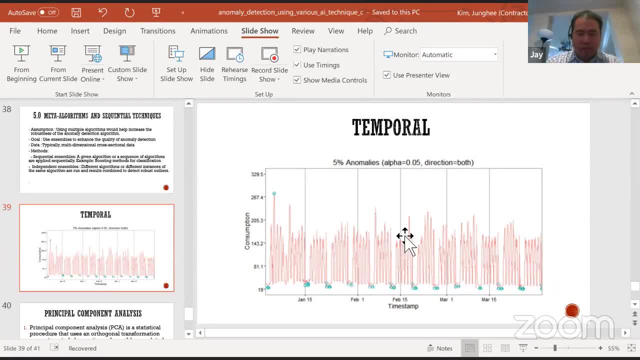 out of the main main, the plot, right. So this one might be, we can think maybe- anomaly, because it's, it's very, very, it's higher peak, much higher peak than any other peak in the pattern. 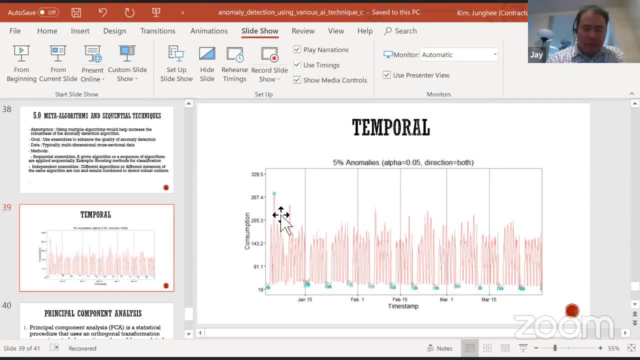 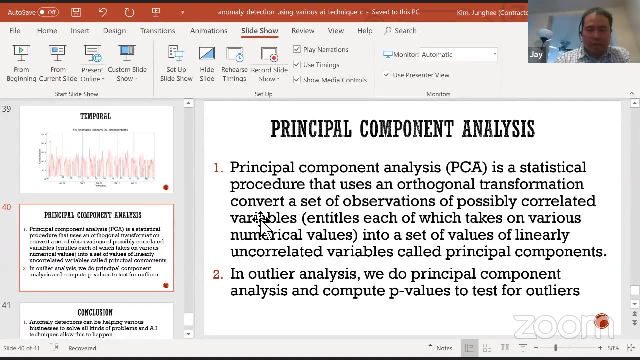 So yeah. So maybe you can think that one is anomaly Again, but this one can be something else, So we have to be careful. And another one is called a principal component analysis. It's called a PCA, So it's very similar to autoencoder. 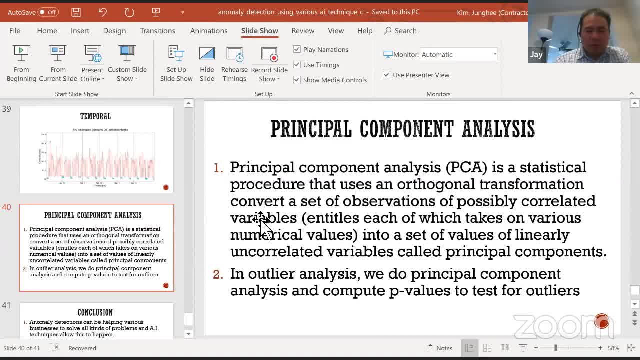 but this one is not the deep learning model, It's not the neural network. So but the you can see that the PCA is is kind of you know it's checking everything in. so the linear, we actually put a linear and then try to get the. 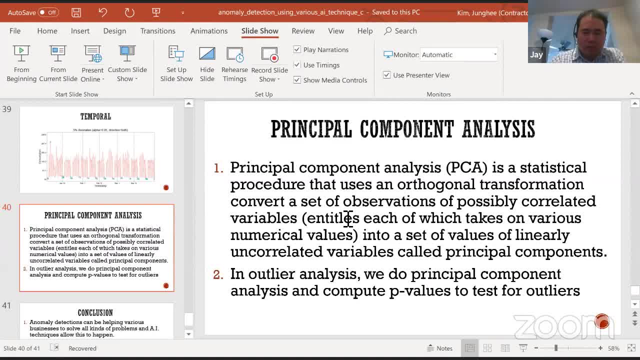 the distance between the data point and the linear, And we actually convert that correlation to the uncorrelated variables, It's, it's called a principal component And then with that value we can actually plot in the two dimension, or two, two dimension from the many. 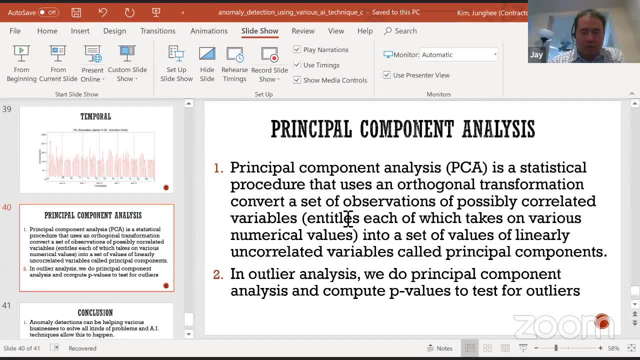 many different features. So, for example, from the 100, the dimension to- maybe you can do the PCA to two dimension or three dimension, But we can actually choose it So we actually get the information factors, information values from the many different. 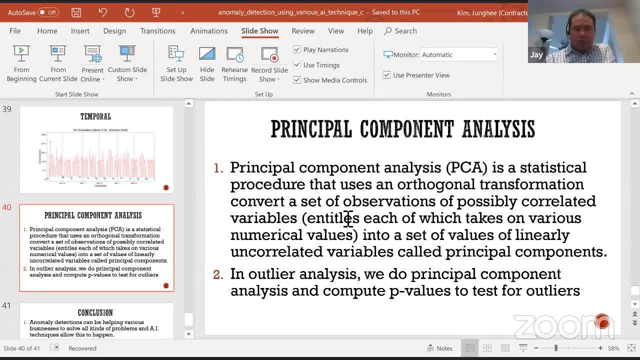 the features, And then we can choose the two dimension, because the two dimension, two features, has the most of the information, So we can actually cut it off and then we can just plot it into dimension and see how the each features the cross. 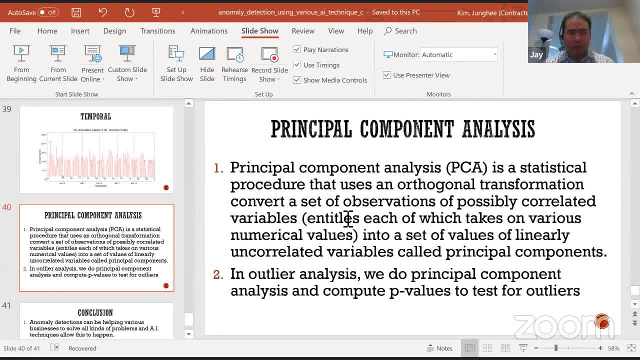 cross each other, kind of So. so we can see that, like some clustering or like some, which is a which features are close to each feature in two dimension. So it is used for the dimension reduction, But so it's similar to the clustering method because we 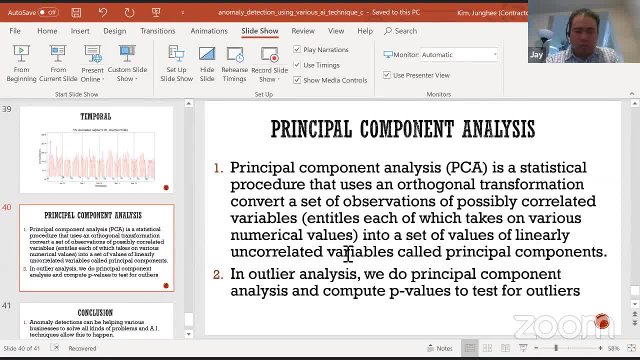 we reduce the dimension to two dimension from the many dimensions And then you can see that if some data point far away from the main data point, then that means we can doubt that as our layer, our layers. So it's, it's a kind of technique for dimension reduction. 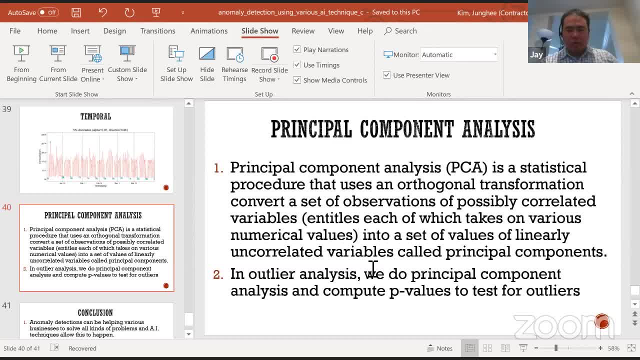 And then we- we saw the earlier before- the auto encoder has can be used as the principal component analysis. So you can see that in the middle layer we can plot it in we, we, we just dimension and compressed join. 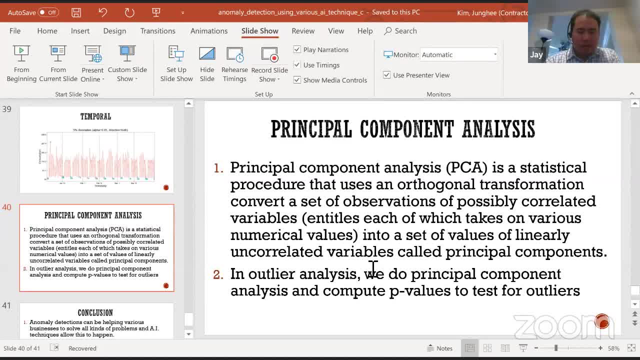 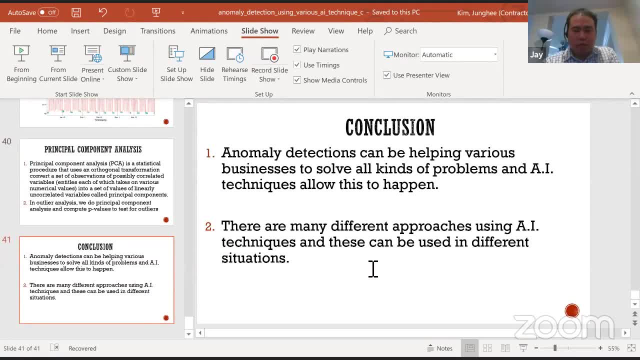 So those can be similar application as the PCA. So yeah, as conclusion, so anomaly detection can be helping many different businesses and can serve for many different problems And the AI techniques is really useful To to serve those kinds of problems With a manual prob. 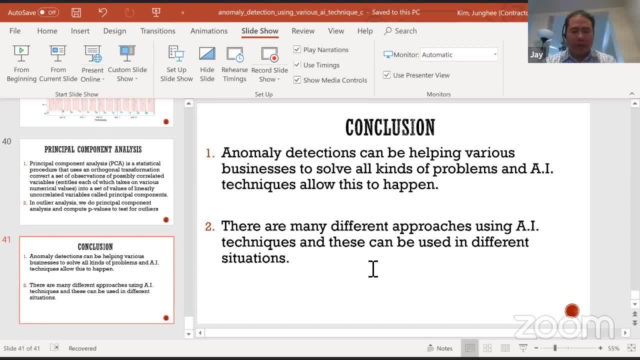 manual way, it's very hard to actually detect those kinds of things, but with the AI you can automate it, And there are many different approaches in AI, So if you know what kind of techniques you can use or in what kind of situation, 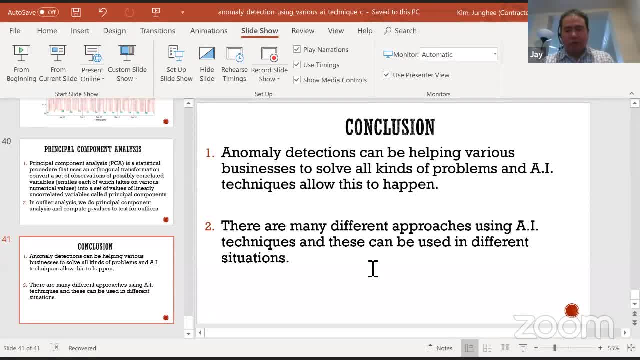 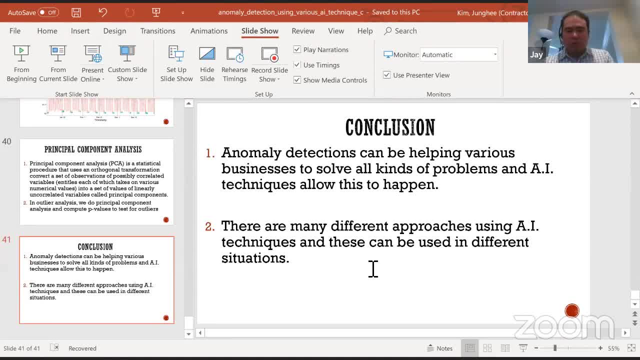 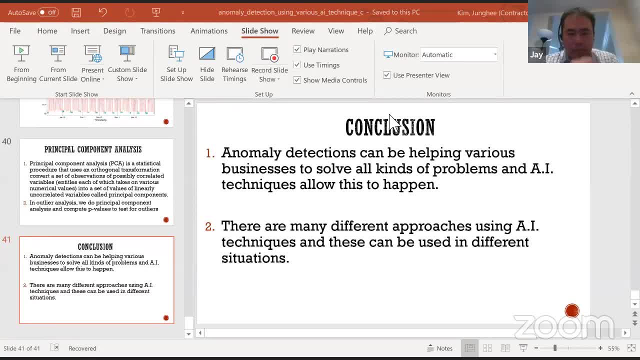 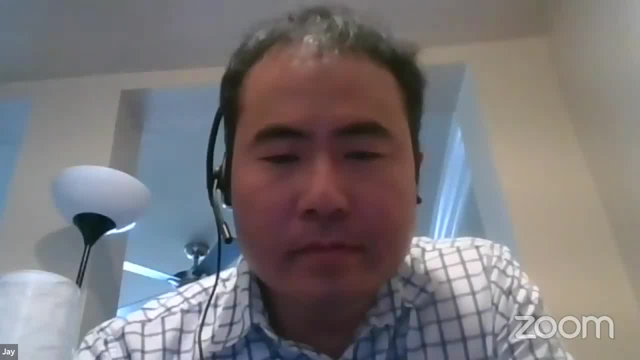 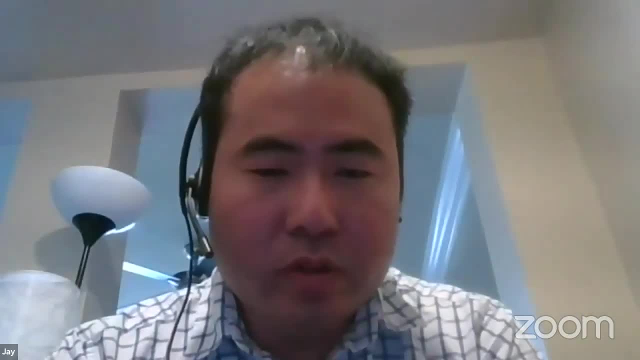 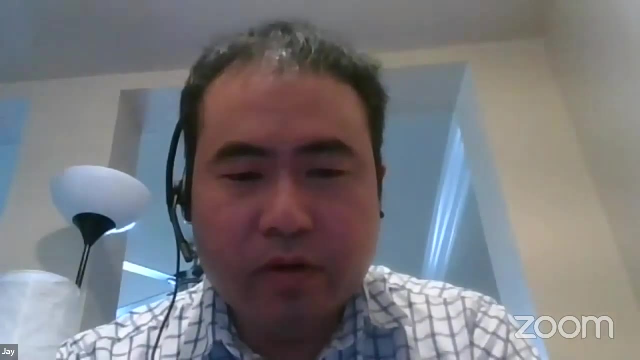 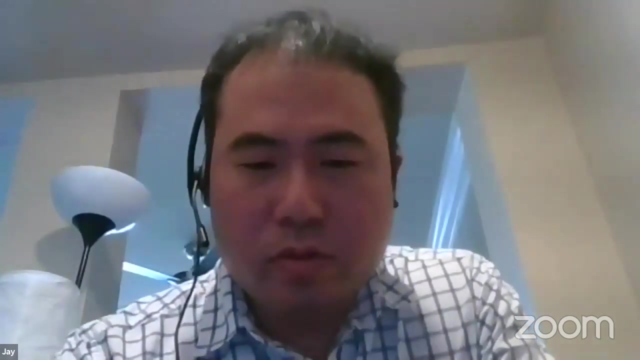 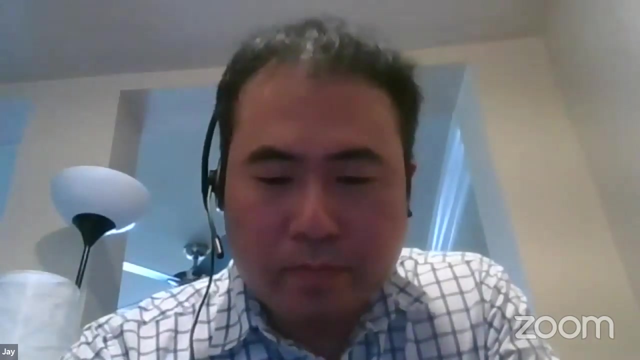 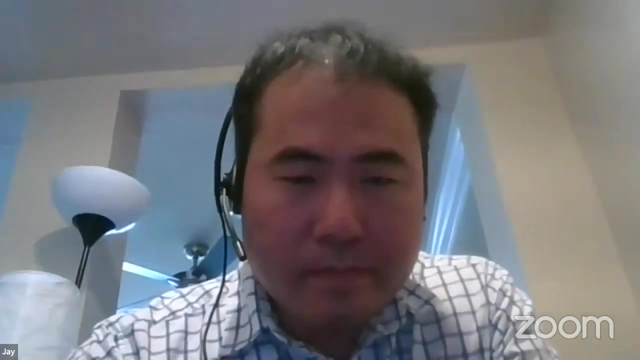 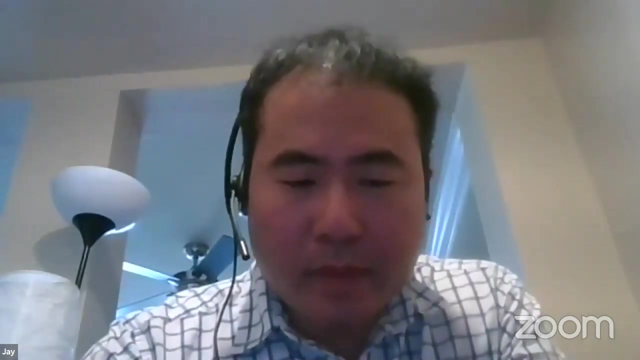 so so Okay, One person actually asked some question: What do the top and bottom bars in the box plot indicate? If they are max and min value, why would anomaly be outside the range? Okay, So I think it's asking about the box plot, right? Okay, I will share the screen again. 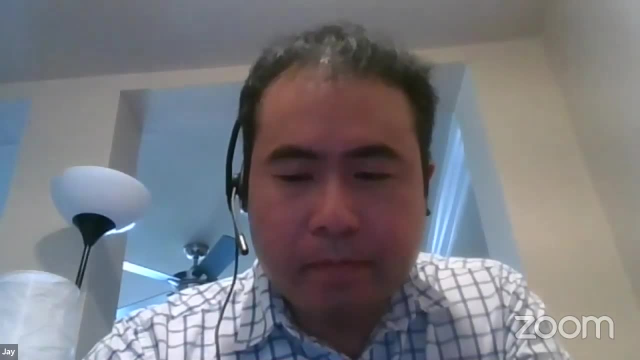 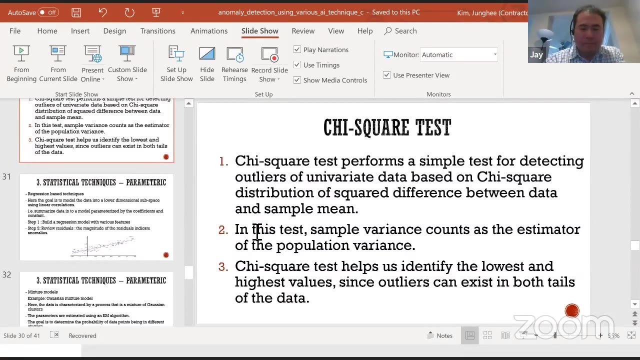 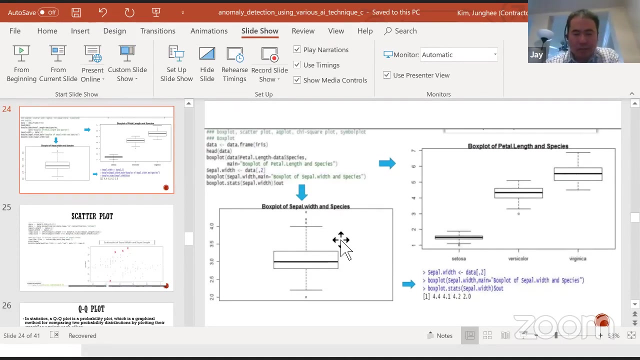 Okay, I think the question was this one, right? So box plot it's like some max and minimum value, the outlier here. So okay, And then this is a minimum value and it's the quarter, first quarter, And this is the last quarter actually. So that means third, third, fourth, three-fourth. 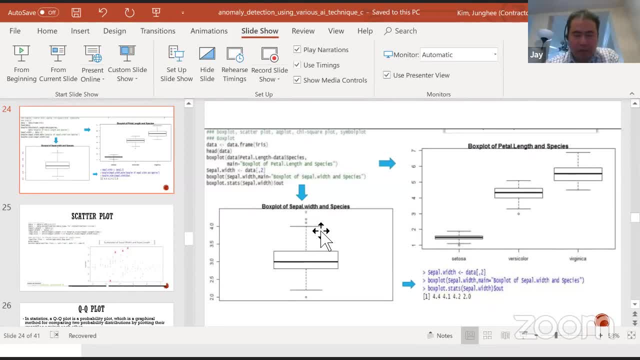 And then after this or so, after that is the max, And so we can just say that it's max. And then this is a minimum means means here like the third, three-fourth of the data is all here, And then very few are actually out of the box, out of the min and out of the 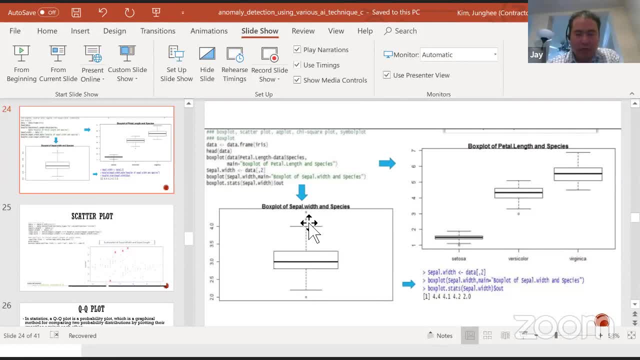 max. So we can see we can actually doubt this anomaly, but it's clearly an outlier. And then another question: Are there multiple different algorithms for principle component analysis or just one? Okay, It's a good question. There are many different, so PCA is just a. 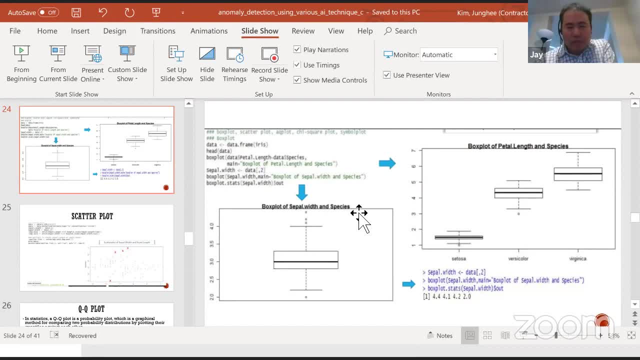 general term. Okay, It's a good question. There are many different, so PCA is just a general term, But there are different. we can actually apply the PCA to many different ways. So, for example, there are many different researches going on. 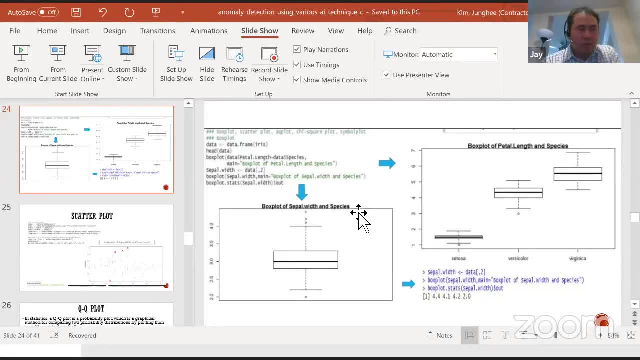 But PCA. this is some commercial PCA that we can use as a library, But in the research we actually develop more our own algorithms. So update, upgrade, more specific usage. So it's not only one. There are many different algorithms. you can actually use it or create it or develop it. 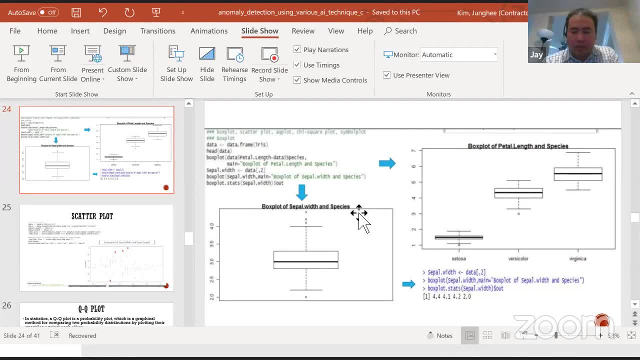 So there are many different ways. Then another question: In integration-based outlier detection, as the outliers are minority, what are the techniques to over-sample the minority level, Like the SMOTE, which can be a good prediction weight? Okay, it's a good question as well. 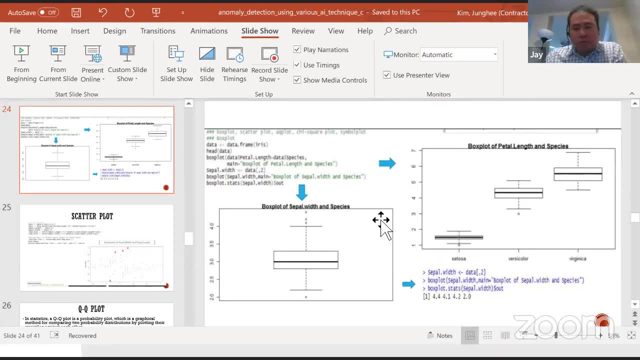 So in the regression- not actually regression but the classification- I think in my experience classification needs a lot of the labeling And then the anomaly has a very few And then non-anomaly is really a lot of data. 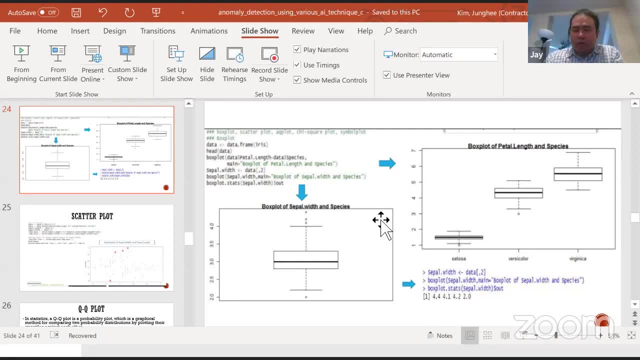 So the unbalanced, imbalanced problem is more in classification problem. So in the case, yes, good way to actually over-sample or down-sample or doing some SMOTE stuff like some synthetic, synthetic sampling. But you have to be very careful because if you down-sample too much, 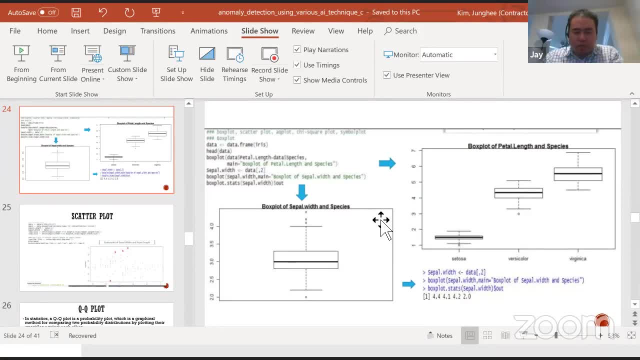 then you can actually we throw away really meaningful data. Then it's not good. Also, when you over-sample- if you do too much over-sampling, then the data we are actually using same data again and again. That means we are over-simplifying. 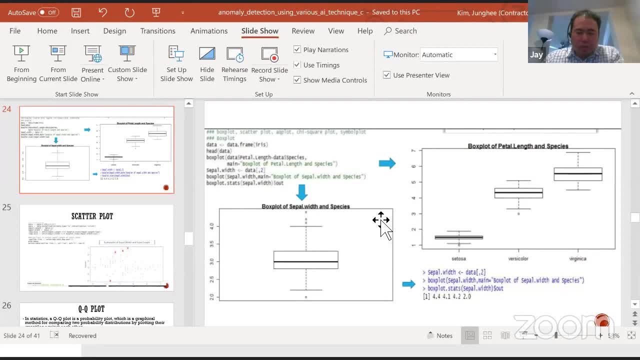 So, and then synthetic is another way, which is actually we create the similar data, but it's not same. Yeah, so they can be actually help, But we have to see what is actually more, what we can actually gain more. 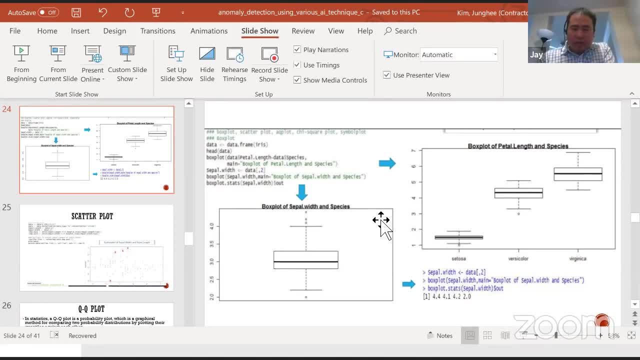 what we don't gain more. So it depends, But I think the synthetic way, like SMOTE, can be. actually in my experience it help a lot. But nowadays there are some more techniques coming up, like the data augmentation right. 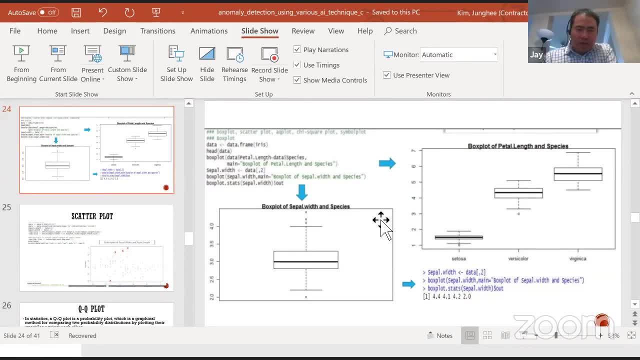 We can actually create some fake image, but it's not very similar to what you have. We just change the angles or we just make the some maybe more specific stuff in the image, And then we, when you train, it's not, and also we actually 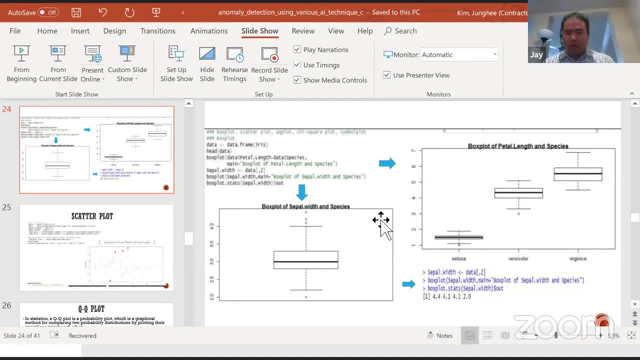 make the like a little bit smaller, make it bigger, So we actually create the some create the more images, more data, more label, data, right, And then we can train that way. So there are many ways actually applied. 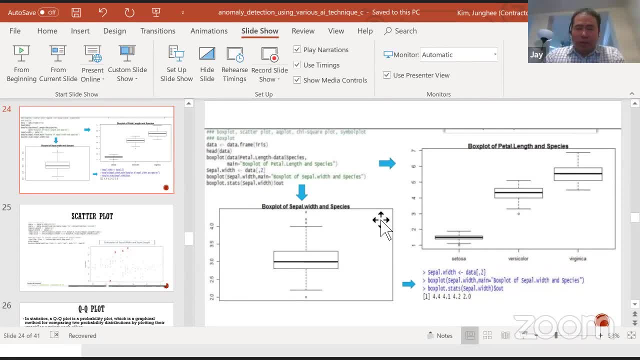 And also autoencoder- or I was working on the variational autoencoder- You can actually generate some data out of the neural network. That can be that data can be used For label data as well. So there are many, many ways. 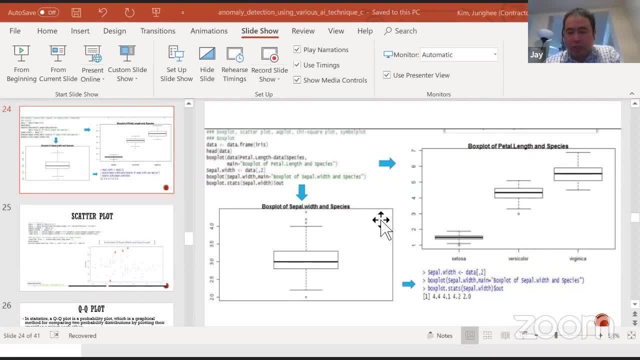 Okay, another question: When do you determine the outlier is anomaly? Is there a situation that the outlier may not be anomaly? Yes, yes, So it's a good question. In the business there are many. yeah, we can actually detect the outlier very easily, right? 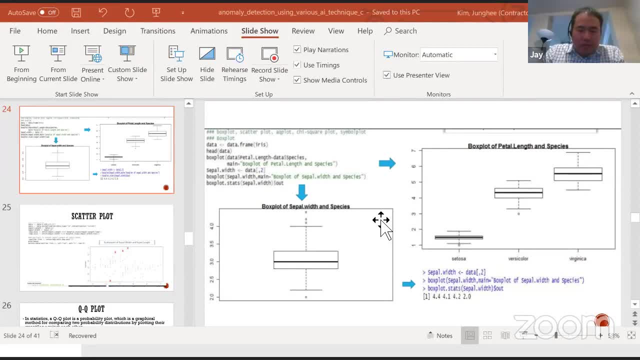 Some, some, some signals are out of the main signal, But there's not always the anomaly. So so when I was working, when I'm working now, after I, I detect the outlier, I, I, I have a meeting with the like business, business people. 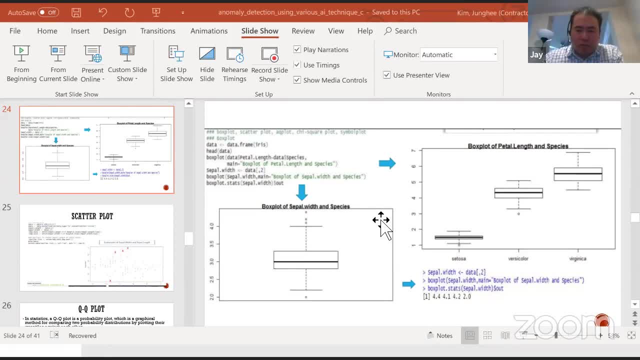 And then we compare. I show them the what is the outlier looks And they actually verify. They can be actually anomaly Because they know, like what is the value of the company, What is the business, So they can tell this is useless. 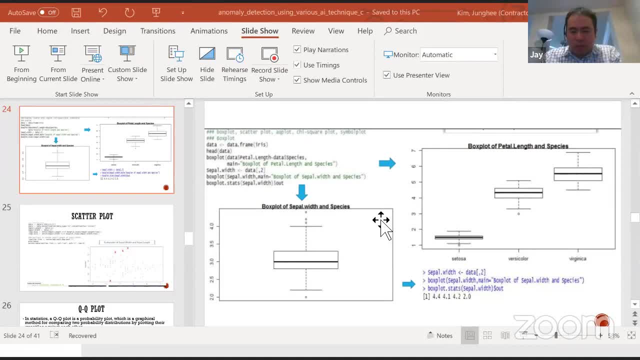 Or this can be actually something they can use for their business. So it's very important that talking with the business folks, So they and we actually communicate And then they can actually give the feedback. And also, if you something, if you find some anomaly, good anomalies. 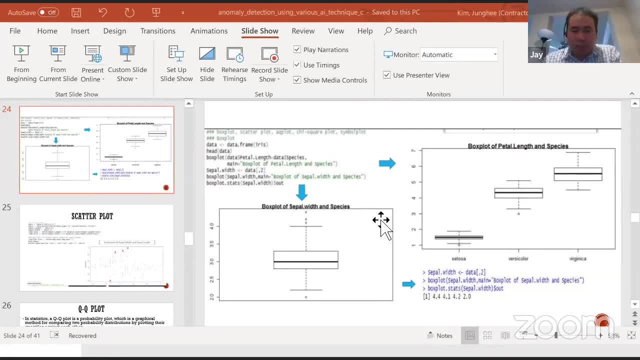 then they can actually use it their way in their business. Okay, So another question, Following up question: Sorry, Okay, Does oversampling always work? Otherwise, what other technique do we do we have? Okay, Yeah, I think I already explained, right. 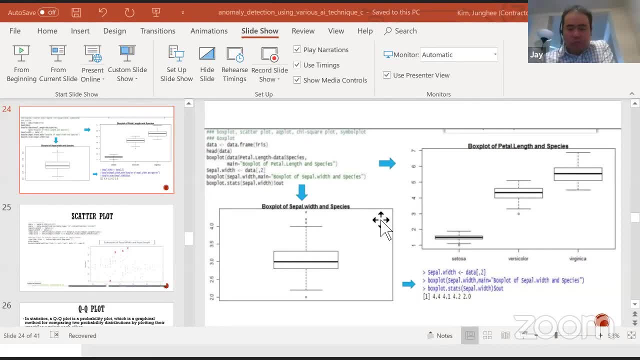 So not always oversampling, Oversampling is not always working. So, depending on the situation, we have to use undersampling or oversampling, Or synthetic way or data augmentation. There are many different ways, So it depends. So we have to see, like what kind of problems we should be having. 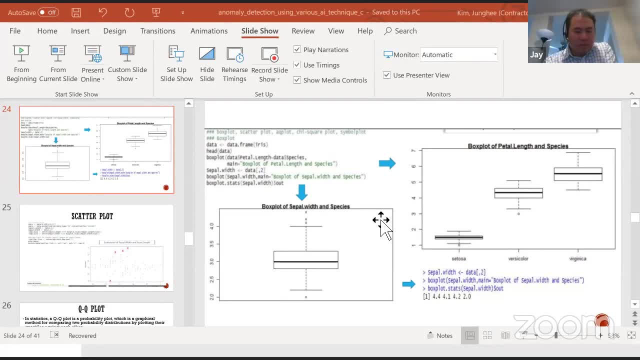 So, from my experience, don't oversample too much. Maybe one-third of oversampling, Maybe one-third of the data, Maybe It's okay, But more than half, then it's already. you're already too much overgeneralizing your data. 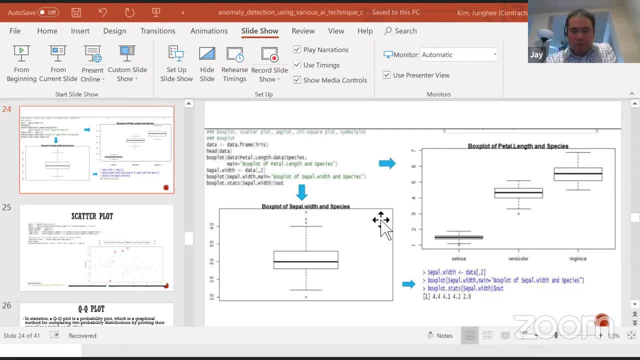 So you have to be careful if you do oversampling too much. So yeah, So be careful. I did not understand your explanation of the top of the bottom bars of the box plot. The top bar and top box is one-fourth of the data in top of the box. 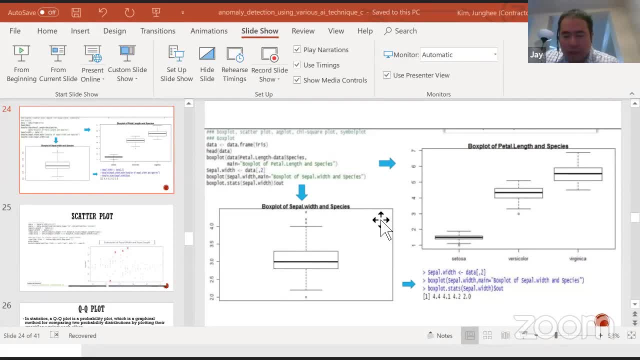 Line in one-fourth of the data. So on the bottom half, then that's four multiplied by Okay. So nothing would be considered an anomaly, Okay, Yeah, I don't, Okay, I think. Okay, I don't actually get this question very quietly, but let me see. 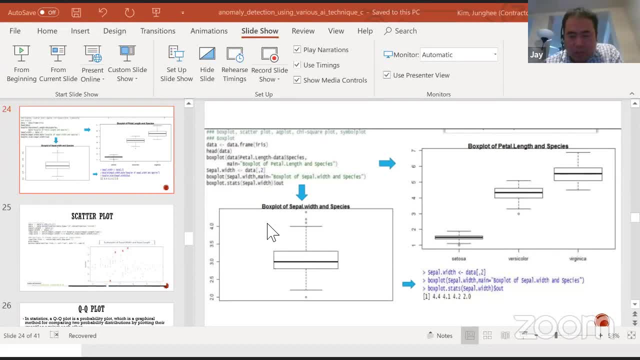 So this button, Yeah, So the max value is one. Okay, One-fourth of the data is actually top, And then one Okay, From the median right Median And then one-fourth of all the data here. 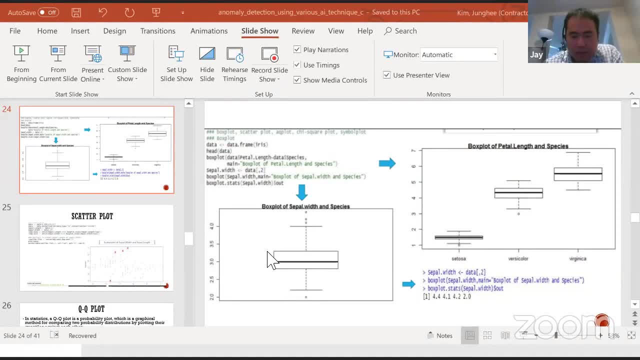 Okay, So the whole bottom is actually out of the bottom. Okay, So the bottom side is out of the bottom. So now we have a quarter and a quarter, and then this third quarter, and then this is actually out of the day. 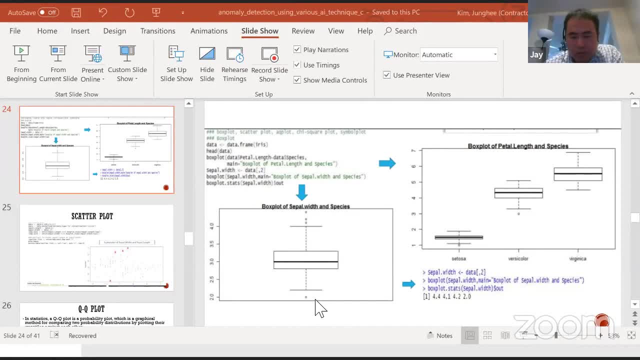 And then this one is same thing, It's a median, The one one-fourth. So our anomaly will be: it's not anomaly, but outlier will be out of this mean and max value. so you can think that way. Okay. so another question: Could you explain more about PCA being used along with the p-value for outlier detection? 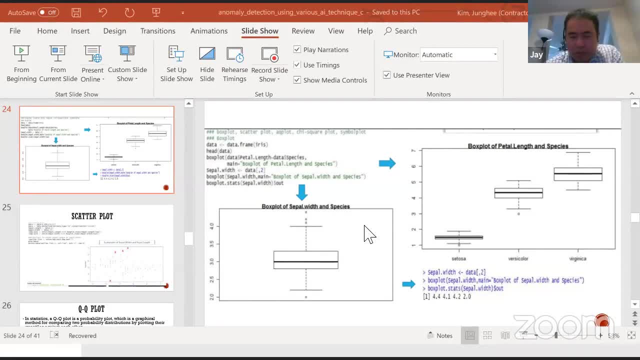 How does dimension reduction help? Okay, I think the PCA is not. you cannot. I mean you can use the p-value with the PCA together, but more commonly you can use this clustering method. So just reduce the dimension to two dimensions and then you can actually cluster it in that dimension. 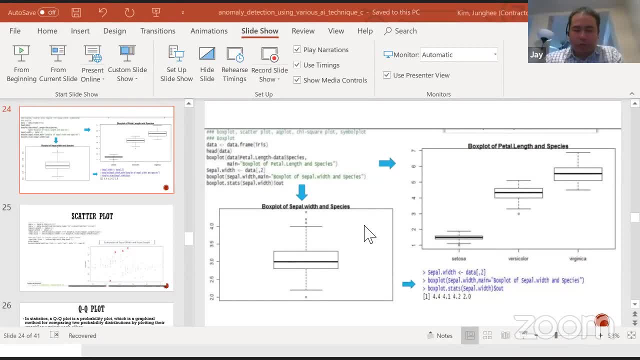 So some value will be out of the mean and max value. So you can think that way. Maybe you can detect the outlier. that way, The p-value is more for distribution. You can actually. yeah, so it's a little bit different, yeah. 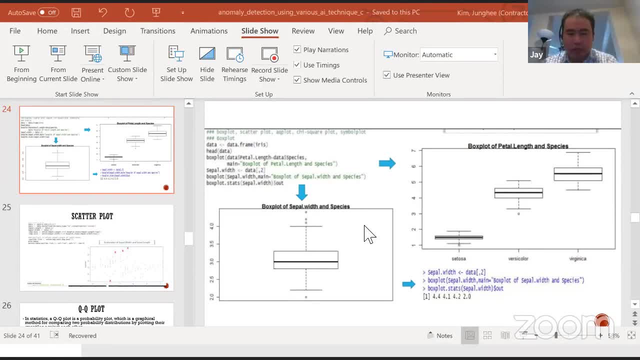 Okay, so any other questions? Okay, yeah, thanks, Hello, this is April, I think we got all the questions And I would like to say thank you for your time and this great presentation And thank you everyone for joining us today.